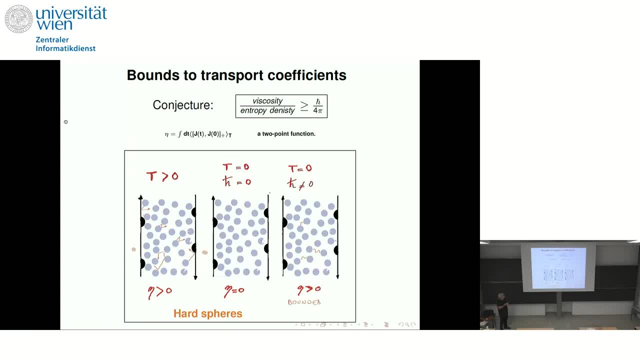 of this. So I want to understand the viscosity of this. So I want to understand the viscosity of this thing, And viscosity is the transfer of transverse momentum And, of course, this is because the particles get some momentum from one wall And because they move. they. 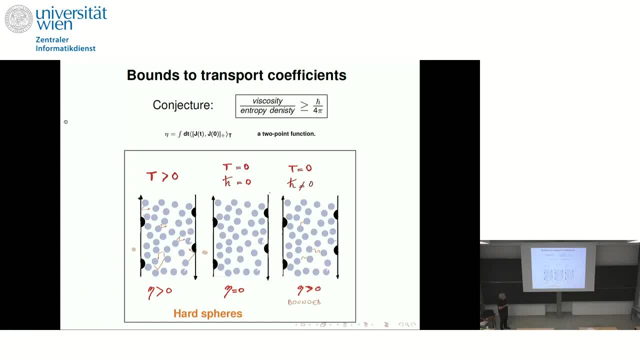 take it to the next particle with which they collide. And you see that this process is going to be in a way, proportional or grow with the temperature, because the way that a particle has to go and walk to the next one and give it its momentum. 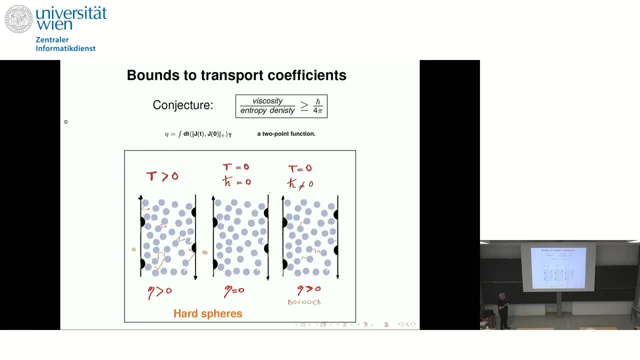 It depends on how fast it is moving. And so when you are in a classical case and you take the temperature to zero, so particles are really not moving, except, well, they are slightly reaccommodated by this motion, But to the extent that this remains a zero. 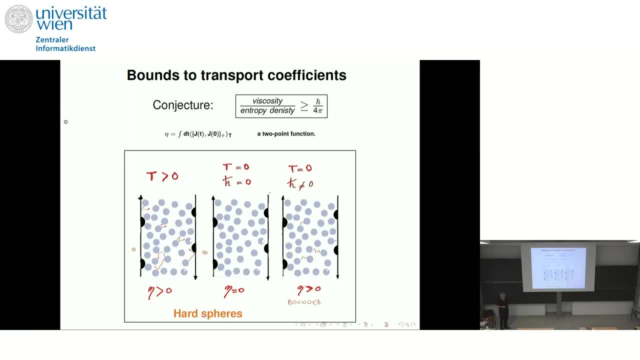 temperature situation. the viscosity drops down to zero. However, if now I switch on the quantum mechanics, I'm going to have to go back to the quantum mechanics and I'm going to have to go back to the quantum mechanics. What happens is something else You can see. 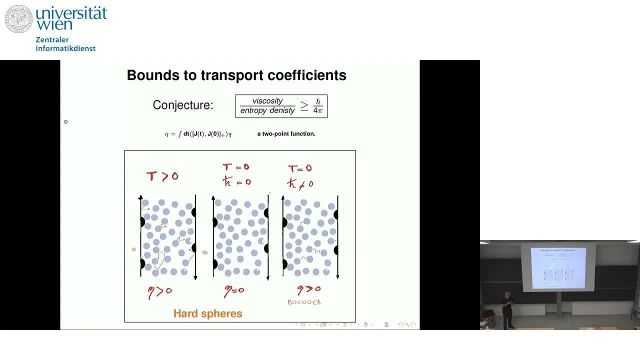 it from two points of view. One is that two particles do not want to be very much together because they don't want to squeeze a quantum wave beyond de Broglie length. We know this because we all solve the square well, And we know that when we squeeze it, the energy 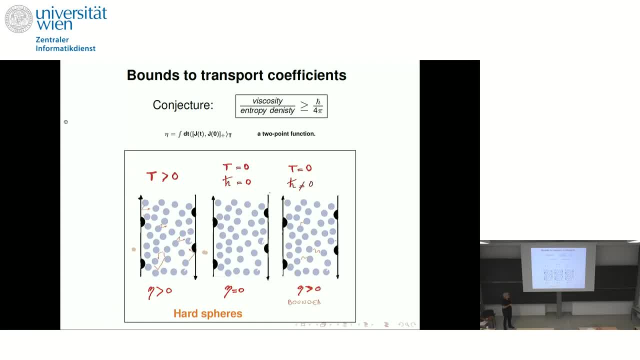 goes up. Another way of saying the same thing is: there is a zero temperature kinetic energy. So the idea, this very simple example already gives you an idea, And there was a conjecture that originated from string theorists that if you divide the viscosity by the entropy, 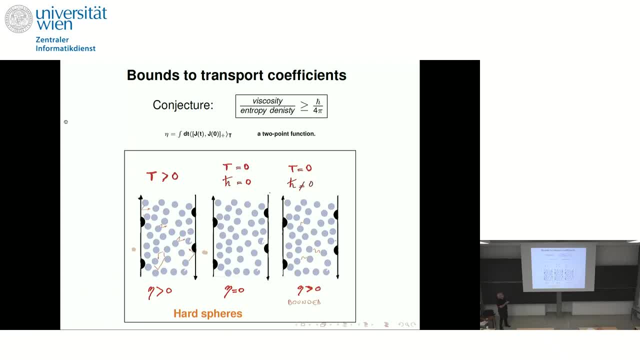 density. this is always going to be bigger than something. This something h bar. well, no, let's wait a second to say what this something is, But OK, so why these people found this magic- And I will come back to this again- is because the models that they had for black holes 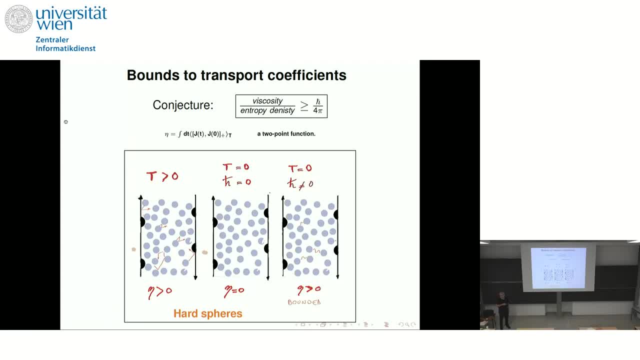 which are very toy models, saturate this bound. So this game is played on two levels. You want a bound and then you're particularly interested in things that saturate it. Things that saturate are things that are related to black holes, holography and what have. 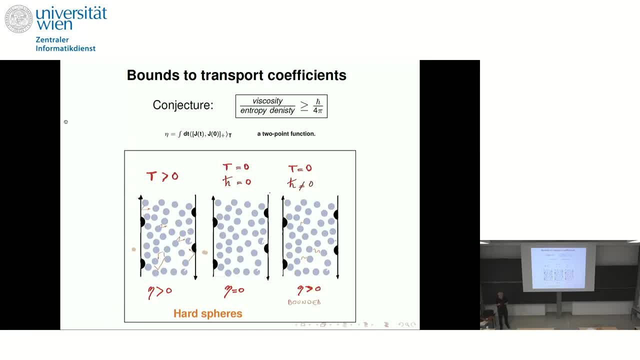 you. But if you have- I don't know- plasma or something like that, or even a solid state system that goes close to the bound, then you can start dreaming of maybe something. Holography is going to help me in this subject, So it is a symptom. 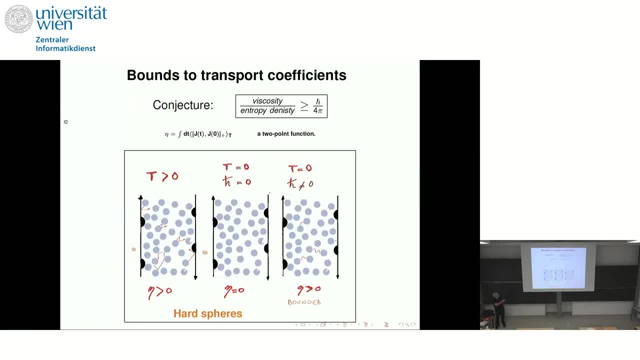 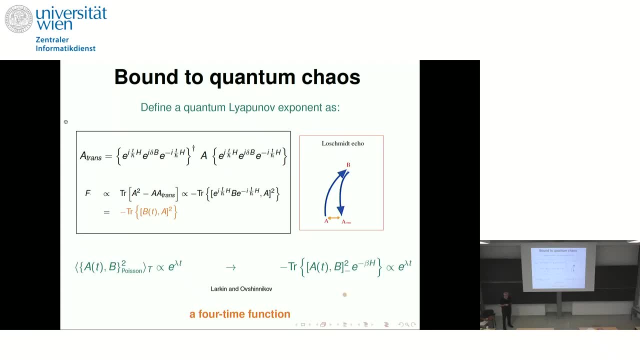 Now, nobody was able to prove this except verify it, And I will come back to this. but it's not even clear if it's true, There are counter examples, but when you talk to people, some of them don't like the counter examples, And OK, Now, this was the situation until. 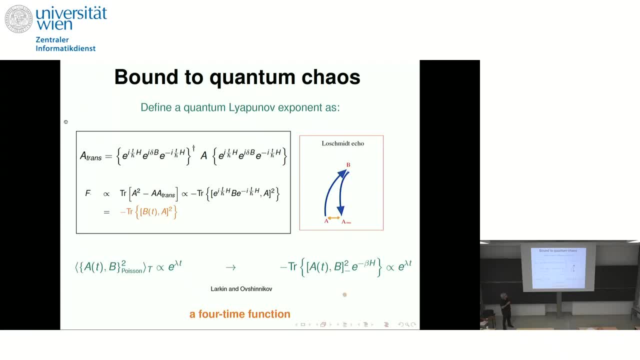 I didn't put the name, but Maldacena, Schenker and Stanford decided to look at another thing where a bound could possibly exist, a quantum bound which is a Lyapunov exponent. So we have to first spend a minute defining a quantum Lyapunov exponent. We have no trajectory. 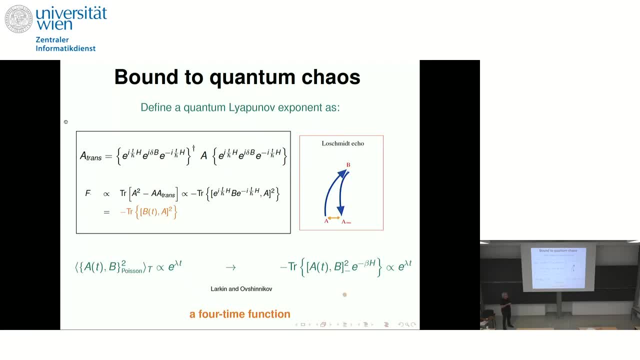 so we have to think what we are going to do. This was done for us by Larkin and Ovshinikov many, many years ago, But the best way to put it is the following: You have a packet, or whatever You evolve, and now you kick the system and evolve it back. You can do. 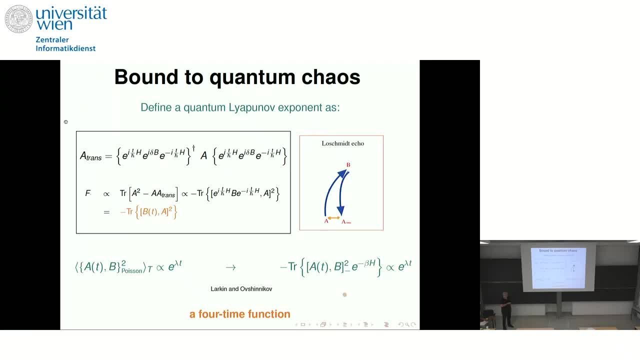 this in the computer and even in some experiments. This is called the Lashmiteko, And you realize that the difference between what comes back and what went is a nice definition of a Lyapunov exponent. But now you can do it quantum, because there's nothing that forbids. 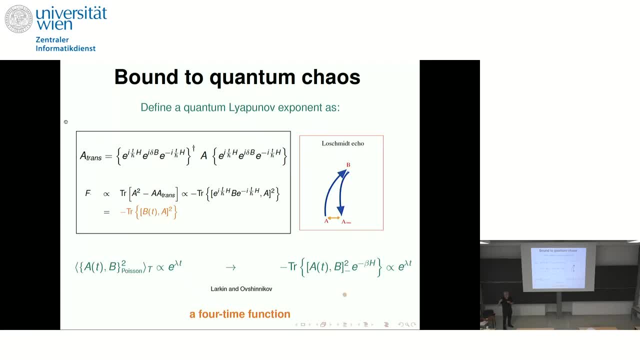 you from evolving kicking and evolving backwards. So here you have a nice definition and now you measure, You do the- this is what I'm doing- A and then I evolve it forward, Then I give it a kick, and then I evolve it backwards, And then I measure the difference from what? 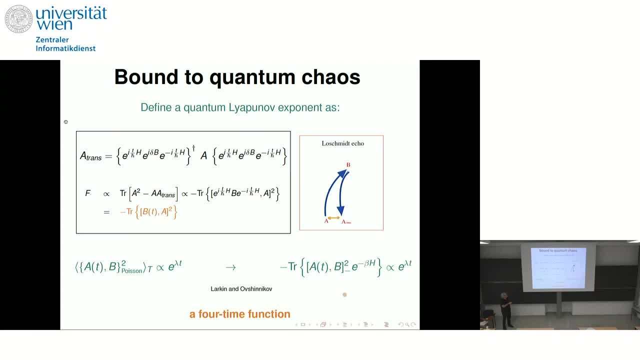 came back. This is a measure of the- This distance here, And you realize that what you get is the commutator of the two operators squared. And now Larkin and Ovshinikov tell you: well, but if you have a commutator, 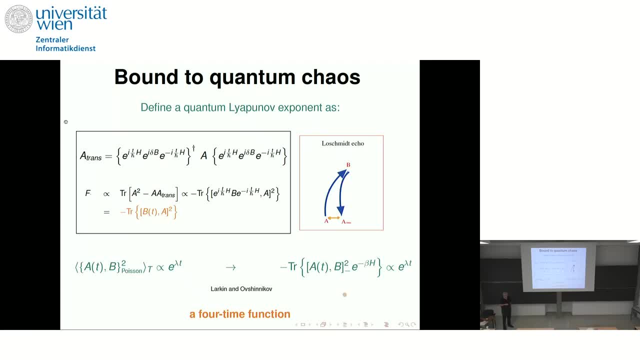 square with a Gibbs measure. now I know how to make it classical, And this is the Poisson bracket square. But the Poisson bracket square is a classical definition of the Lyapunov exponent. So we are good, We have found here a nice definition of a quantum Lyapunov exponent. 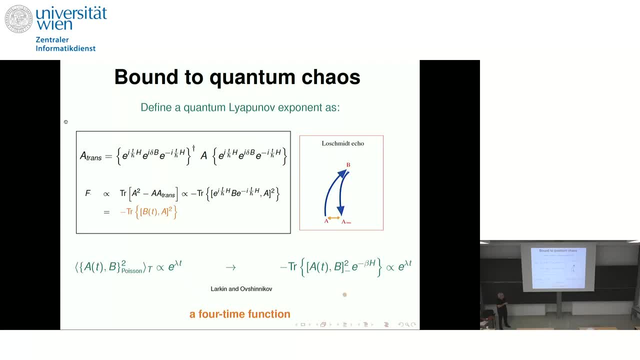 And now, OK, and remark: it is a four-time function because if I do this square, aT, b, aT b, et cetera, et cetera, there are going to be four operators at four different times. 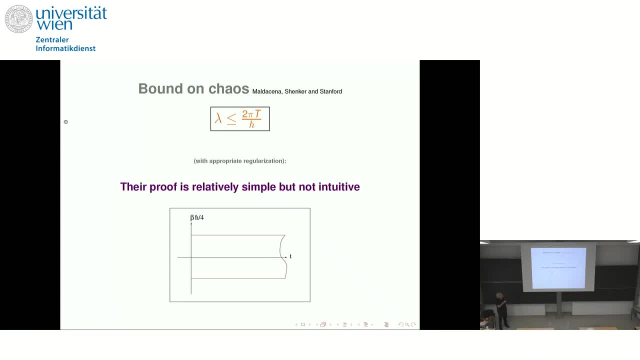 And these gentlemen here proved this bound- that the Lyapunov exponent has to be smaller than this quantity. So as you go to zero temperature, it goes to zero, But as h bar becomes small, larger it also depresses the value. so, and let me say it now and i will repeat it as many times as 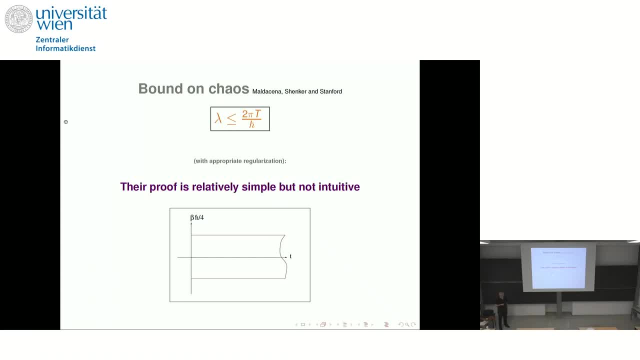 h bar over t is what i'm going to call the planckian scale. it's a thing that has dimensions of time and it's model independent. no, h bar over t doesn't talk about the model. this is the what we call the planckian scale. so basically, what they proved- and this one they did prove- is that 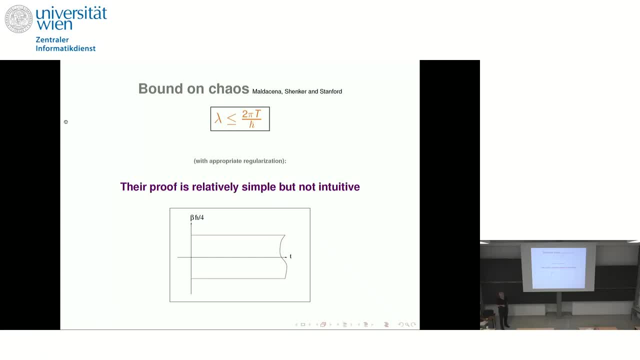 the lyapunov exponent is bounded by the inverse of the planckian scale, under certain circumstances that i will tell you now. yes, this is equilibrium, yes, you are at temperature t and you calculate this commutator squared and you conclude, and you will see this, that this is bounded. i mean the exponential growth. 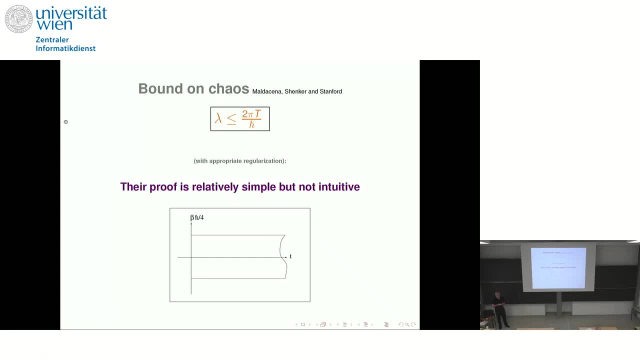 of this commutator squared, is bounded by the planckian scale. okay so, no, no, no. like all lyapunovs in life, they depend very little of of the of the operators. okay, so when you go to the proof, first of all, you say, ah, and this is a nice thing, their models of. 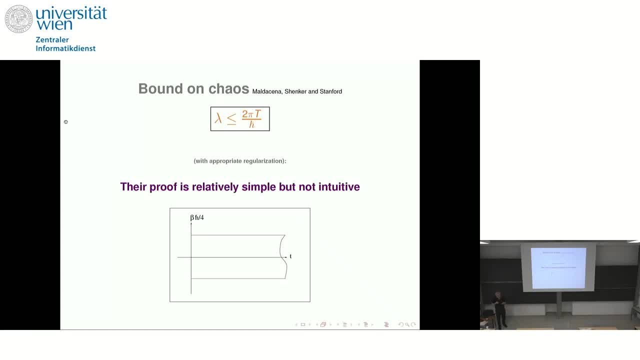 black holes, saturate this bound again. this is why they are excited. but uh, we are excited not for so much for that, because it doesn't talk to us very much, but this: the question is: is this a string theory result? or is it just statmec plus uncertainty principle? and this is what 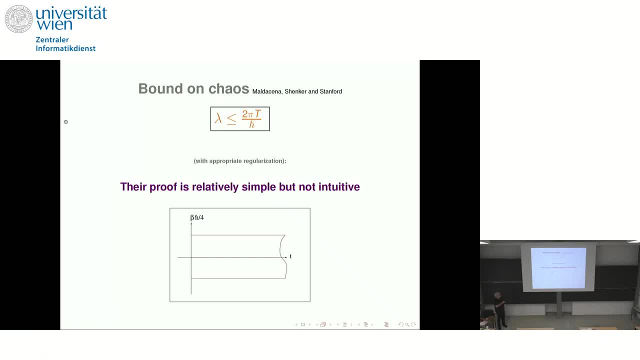 it is so. this is why i'm talking about this here. so the proof uh is: um, you can follow it. it's not. it's one of those proofs where you follow six steps. each one of them you swallow, but by the time you go to the six, you know you're a bit lost as to what was. 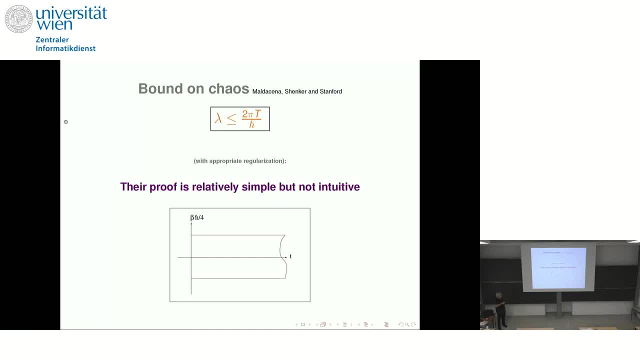 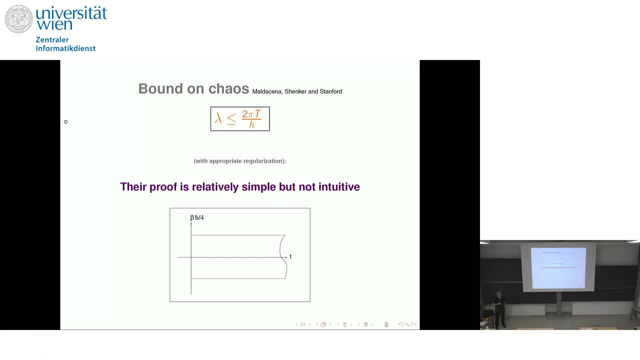 this is what's gonna need dead content. you understand that, uh, so there is no这样 and you're not gonna waste anything by dividing positive and negative part to the population. i think it works. it works very well in our question. and now you uh next question on the one that's right there. you are asked to ask a question of twofold on. 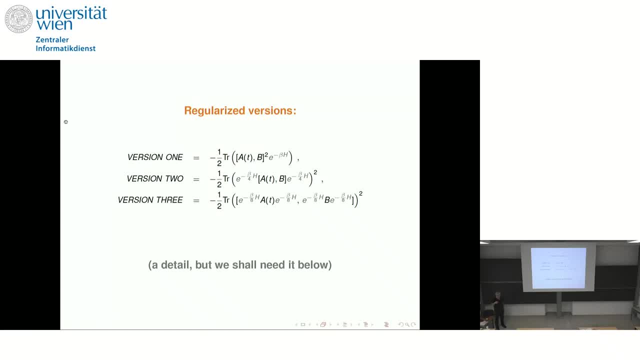 that one, one of the commutators, a quarter, and then you square it so you're chopping up the gibbs measure. it's a regularization, let's say, and this one is another one also, they come classically. clearly they are the same because you can move all the gibbs measure. they commute and you can move it. 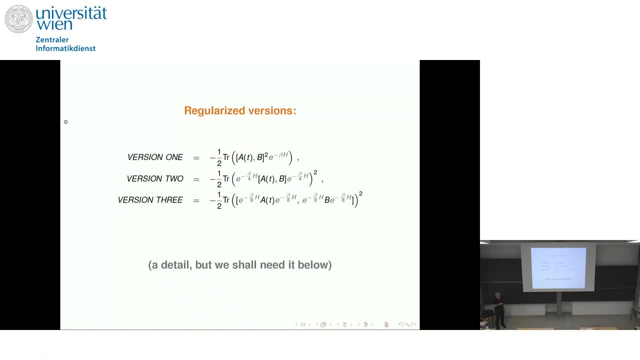 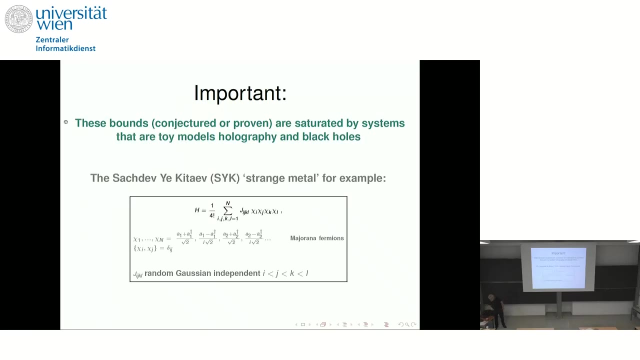 to the end, but we will need version two and version three, and indeed the original proof also needs version two and version three. okay, but let us for the moment say: this is not big deal, it's just two regularizations. okay, um, okay. so again i'm repeating this: um, the point here is that 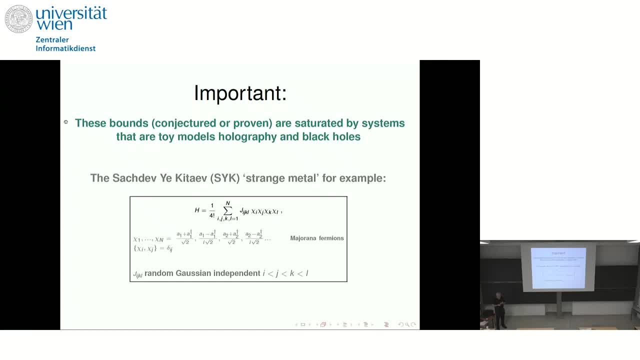 the motivation is that black holes and systems that come from holography, whatever, are expected to saturate these bounds, and this is very important for them. then something amazing happened is that um realized that a very simple spin glass- quantum spin glass- model did the job, saturated the bound, and all that so immediately. because this is a symptom, this model was promoted. 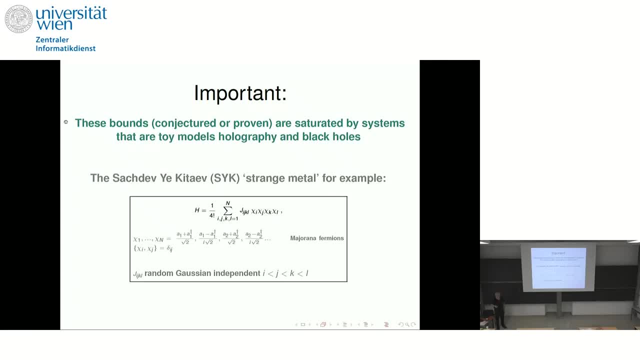 to being a kind of toy model of holography, black holes and what have you with? the important difference that here you know how to calculate everything. so this: it made the field a bit explode, but i'm not going to get into this, but it's an interesting part of the story. 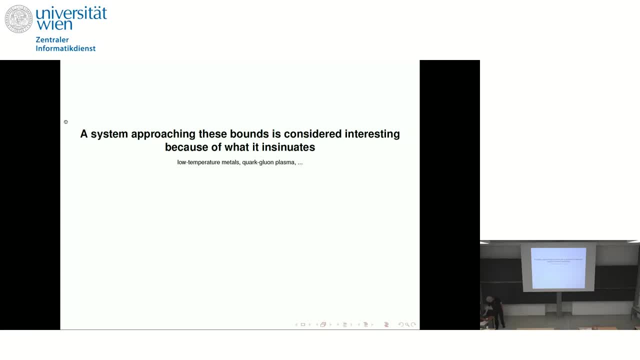 okay, so, once again, okay so, uh, let me make a small detour on fluctuation, dissipation, which was mentioned several times here. well, the classical one, you know, you have the poisson bracket between, uh, two things, and then you relate, you can define this way the 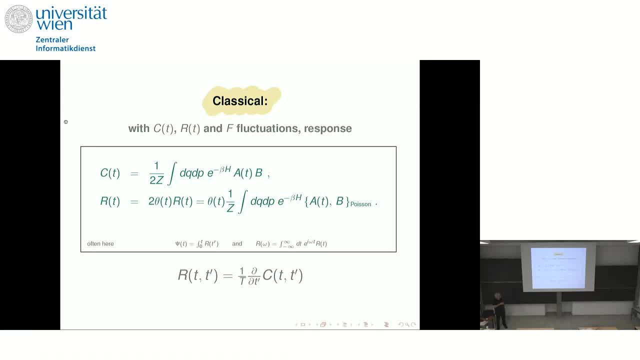 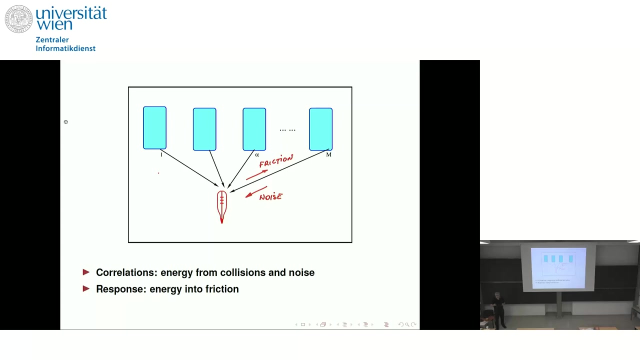 response. you have the correlation, and the classical fluctuation dissipation relates uh the response with the correlation and we will work a lot with the integrated response, which then integrated over time, which then is directly proportional to the correlation. so, no derivatives, okay. so, uh, why is this important? this is not just, uh, some some equality that can help us in. 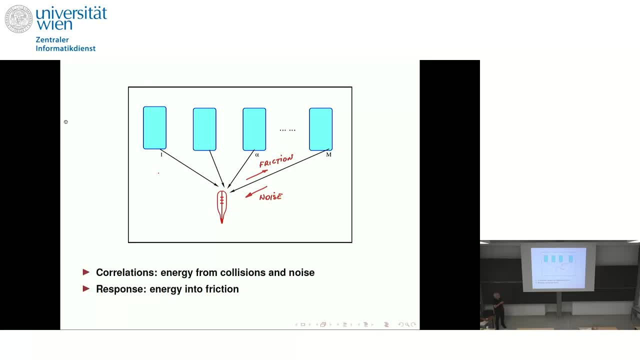 some occasion. this is crucial. if i connect a thermometer to many copies of a system, the same observable in those many copies, and i ask myself what will happen? what will the moment read? i would like it to read, but these are equilibrium system to read the temperature of the system, and. but how does? 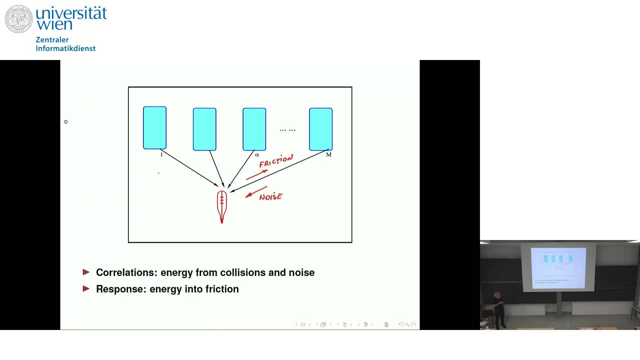 energy. talk to this thermometer. well, noise will move, will agitate the thermometer. thermal noise and friction will stop this. as you see, i am re remaking einstein's argument for brownian particles, and so this balance between these two things work and give you the temperature thanks to fluctuation. 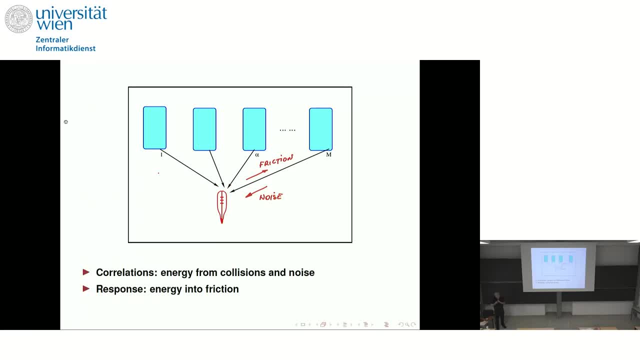 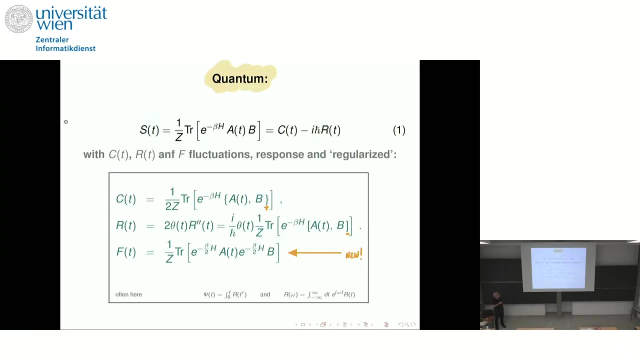 dissipation. okay. so, although- and this is quantum two, because it would be a catastrophe if quantum mechanics broke this, if fluctuation dissipation doesn't work, forget about thermodynamics, that's, that's a point. okay, so now quantum. well, quantum, it's a little bit more difficult, but not so much. 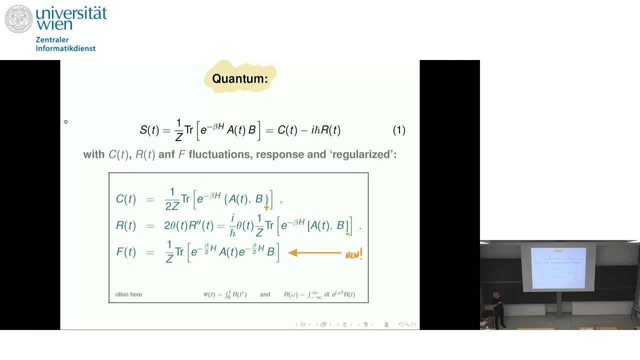 you take the gibbs average and then the correlation- you can show it and argue it etc- is the expectation of the anti-correlator. i'm sorry, these brackets are not poisson now. it means anti-commutator. so a b plus b a, the response is the expectation of the commutator. 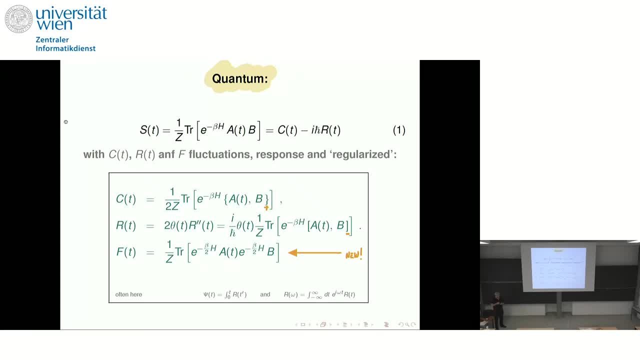 this is what you're taught in and this you can. you can construct it and give a kick to the system and see what happens and and do it, and then a new object appears which will be important for us. it's only quantum, in the sense that if this were classical, i could just put this thing. 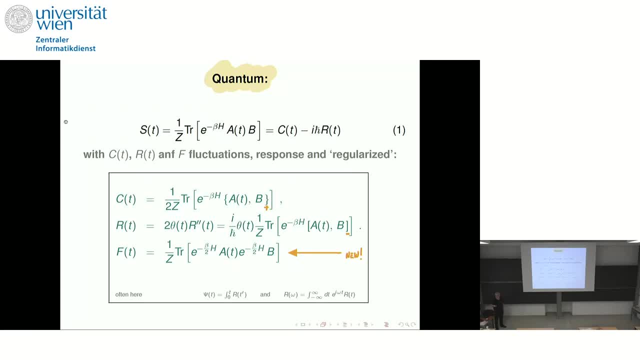 on this side and i will get the same original stuff i had at the beginning. but in quantum mechanics i cannot. this is a chopped measure. you see, i put half and half and this is a very nice object and it will be very important for us. it's it's a purely quantum thing. for the moment it's a 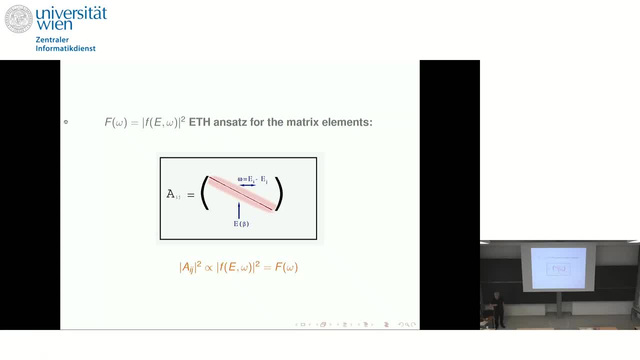 mathematical thing. but okay, um, just for a bit of background, that object there, when you are in a quantum chaotic system and you diagonalize your hamiltonian and you look at the matrix elements of any local operator, it is has a bandy form, it's zero, far away from the diagonal. it has kind of a bind form and indeed the distribution. 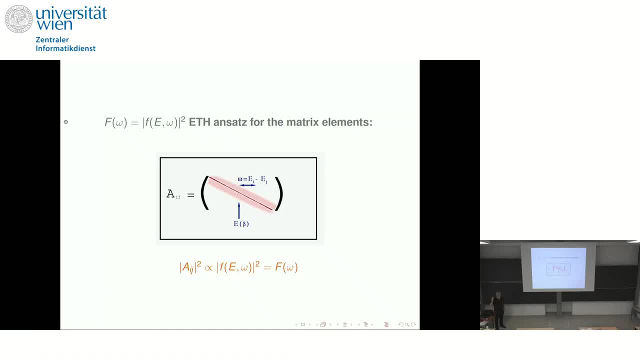 along this band is precisely this f i've defined before, which is: it's fully a transform. so it's a, it it has a meaning. uh, okay, so let me go on with fluctuation dissipation. so you have the correlation, you have the response and now you can prove the fluctuation dissipation theorem, which. 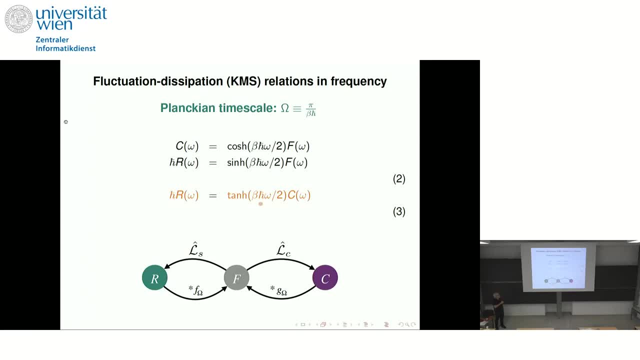 now is similar to the one we all know and love, but with a twist. so the way you find it in books is this one. the response is this: tangent times the correlation. if you develop the tangent, you get in powers of h bar, you get the usual fluctuation dissipation. if not, you have to live with this one. 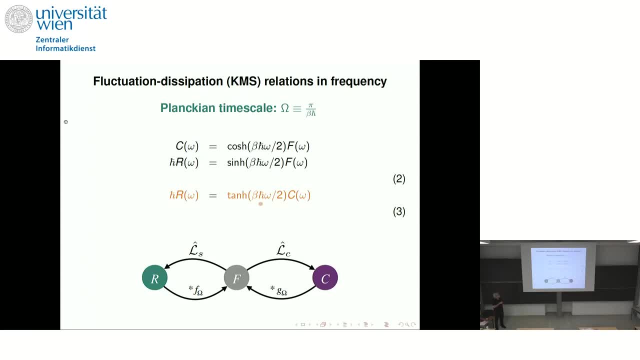 but now i am going to use the fact that we introduce this f function, which is sort of midway, and you can write it in two steps: c is this, r is this. of course, if i divide these two relations, i get this one, but i prefer these two relations. why? because the cosine and the sine are analytic. 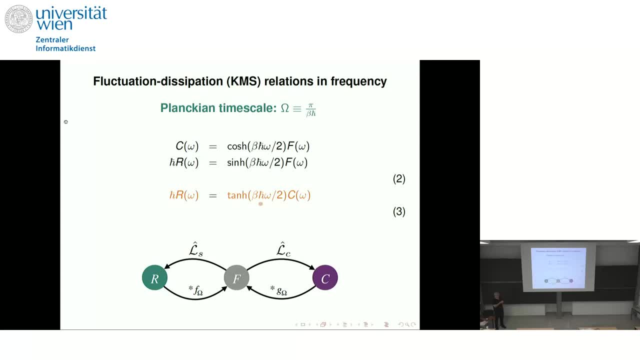 functions rather than the tangent, and it will be useful for us because if you divide the two relations, you get the same thing about the cosine and the sine we have. we are the same thing for us, okay, so yes, yes. well, first of all, the thing i told you about the, the band structure of eth- i came back to, i can 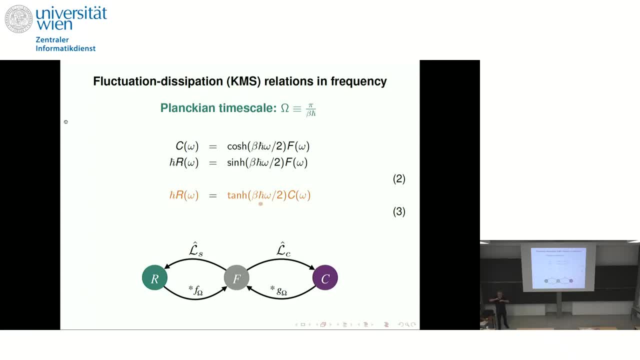 state normalization, but also, you will see now, fluctuation, dissipation, relates. you can write it as: uh, you, you shift the time axis and you say something above and below. that you can write it as, and something below are the same. This is KMS. Well, this line where you put things is the line of F. 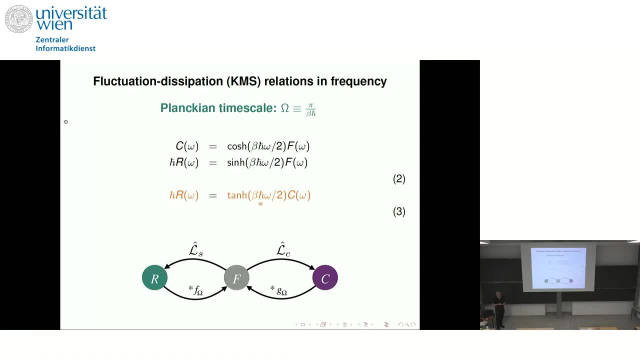 So it's the symmetry that is involved in KMS. Okay, so the usual fluctuation dissipation, as we said, is as a relation between correlation and response. Here you make an intermediate. stop on this function, okay, Why? Because you will see that you learn a lot from it. 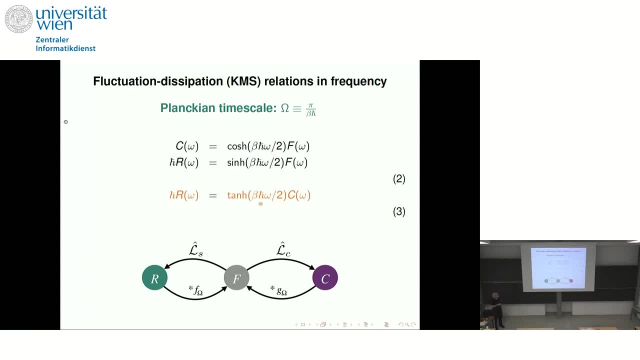 And then you have some operators that take you to one side, to the other, which are, of course, nothing but this. Okay, so let me look at the ones that take you away from F into R and into C. You can write them this way: 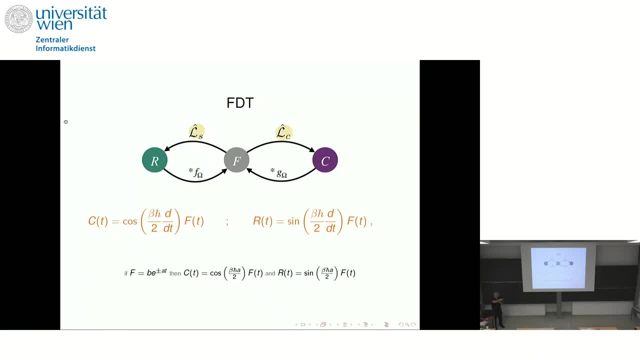 So cosine of a derivative means that you do the expansion, the Taylor expansion of the derivative, and this relates C with F. R is related with F in this way And, for example, you can use this because if F happens to be an exponential, 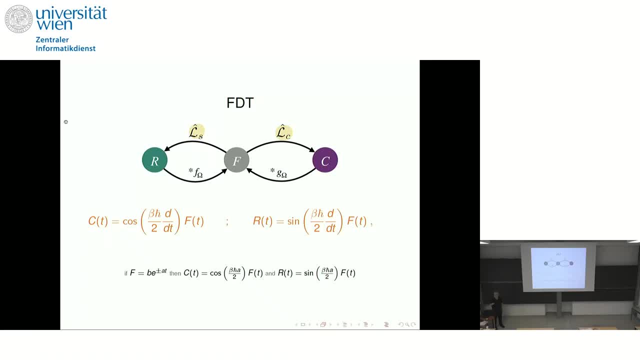 you can compute these successive derivatives And fluctuation dissipation tells you something very simple: that C is now not the cosine of a derivative, it's the cosine of the actual exponent And R is the sine. and you can divide these two so that you find in time that C over R. 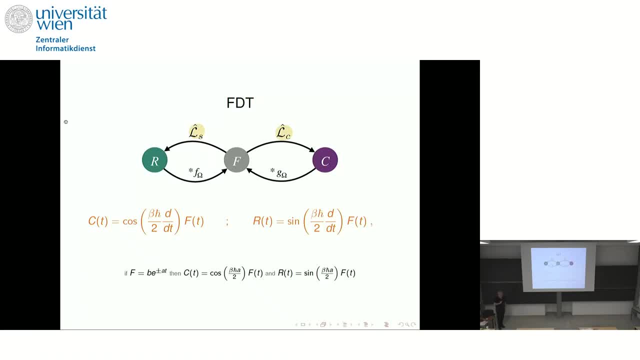 is the tangent of the exponent. So for an exponential this is particularly nice and easy, And you see, these operators are a little bit nasty. in time These are the same as the cosine of omega I wrote before, but here it's a time derivative that is iterated. 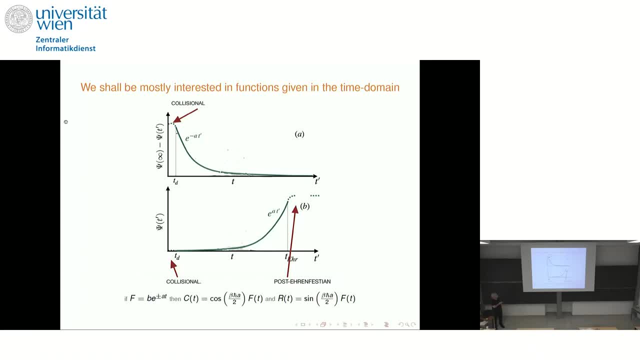 You can do. I'm sorry so for the exponential. as I told you, they act in a very controlled manner and give you a cosine and a sine. simply No cosine, because there is an I in the game, which sort of I don't know. 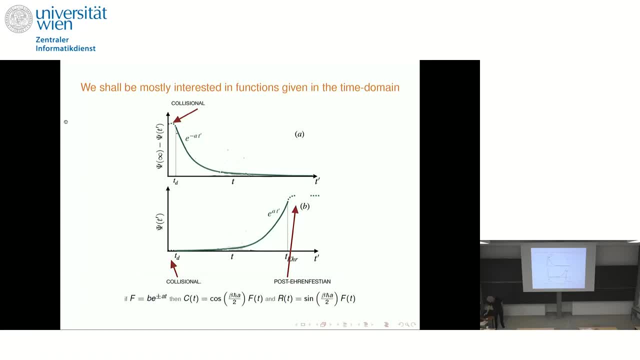 It sort of arranges things and it will be important. Now, the inverse ones are rarely, if ever, found in books, or I would say never. So these are the inverse guys, the ones that and you can show that F is related to C. 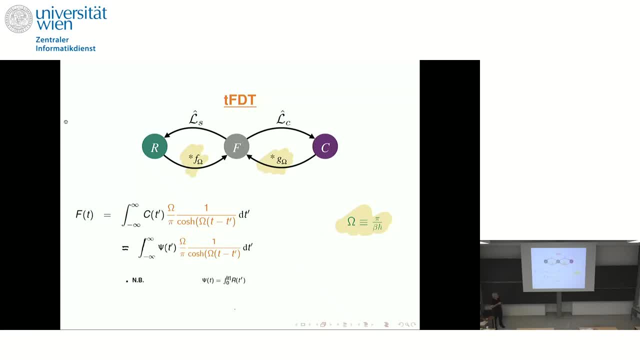 through convolution with this object. here. Omega is the Planckian scale here and in what it follows. So you see you're convoluting with something and this gives you F, And psi is the integral of the response which I told you is a nicer object. 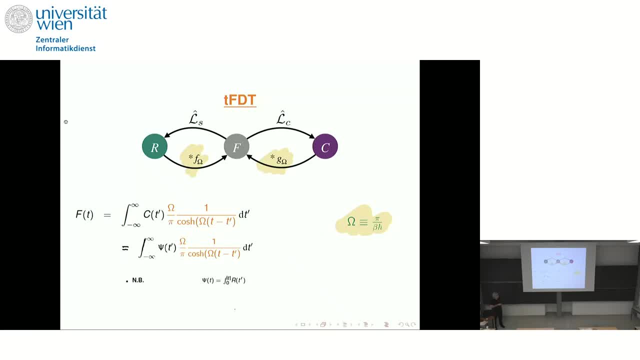 Psi is related to F this way And you see that when the Planckian scale collapses, this is a delta function morally, and you get these identities which are the usual classical FDT. So it's nice and we will come back to this. 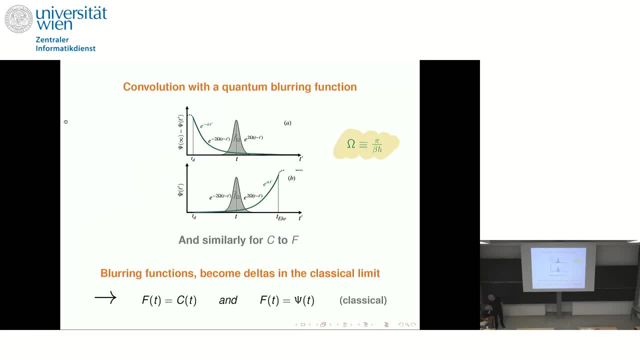 to see these things in time. this way, As this is just repetition, you're convoluting with this bell shape, which is one over cosine whose width is the Planckian scale, And you see, your correlation or your response- integrated response- is going to be blurred. 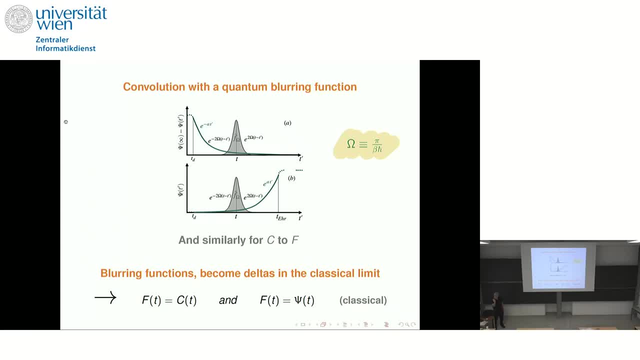 with this quantum convolution, with a thing that has a width. That is the effect of fluctuation dissipation, And they become deltas in the classical limit. Okay, having said this, this is just a recap of the ordinary fluctuation dissipation theorem, KMS. 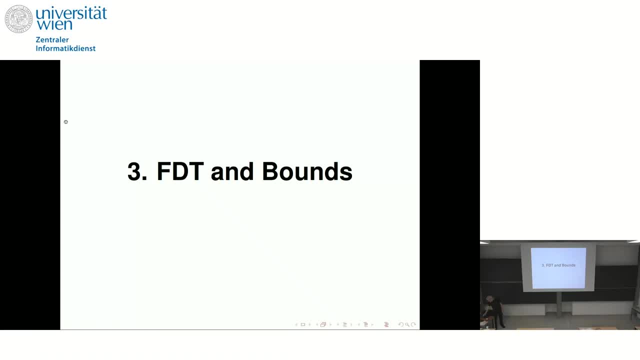 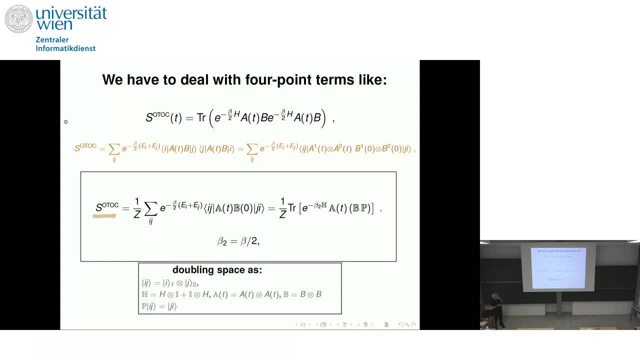 in quantum mechanics, Kubo, Martin Schringer. Okay, fluctuation, dissipation and bounds. Here comes the proof in its easiest form. This was partly done in a work with the group of Ueda Tsuji, and it's a work we've done. 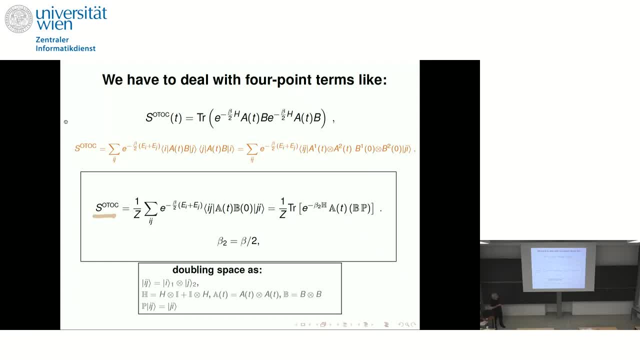 with Laura Foini and Silvia Papalard. It's a reallyению need to calculate things like this. Remember there was a commutator squared, So this is one of the many terms you have, And now this is a four point function. 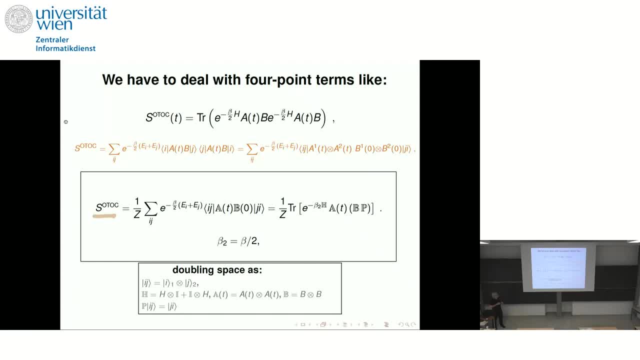 As I told you before, it comes from a commutator squared- This is one of the many terms of a commutator squared- and you have a four point function. But we don't like four point functions because when we talk about fluctuation, dissipation, things like that, we usually talk about two point functions, correct? 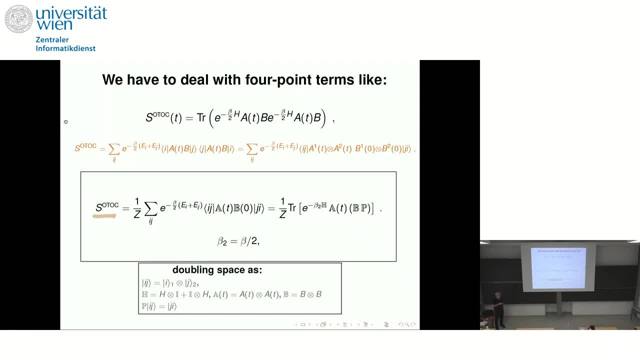 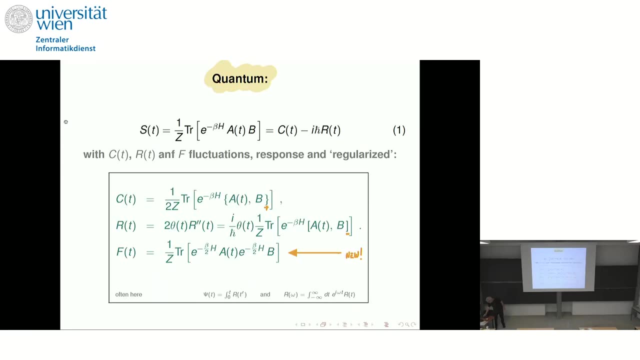 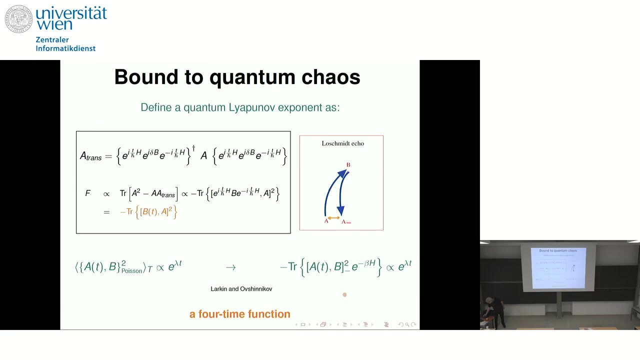 functions. So, yes, Okay, this is just the definition of one of the many terms that come when you develop the commutator here. Remember you wanted to calculate things like: sorry, you had many terms coming from here. yes, This if you develop it's a different square. 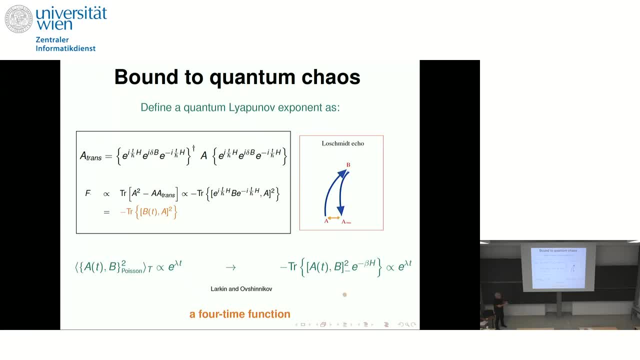 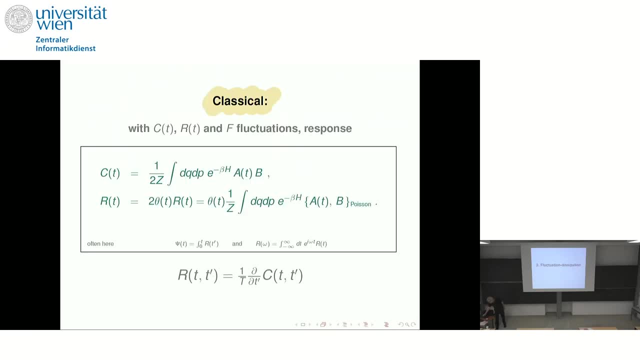 no, So it has four: A, B, A B. You develop the anti-commutator square, So it gives you many terms. okay, One of them, but just to show, I took one of them which I call S. 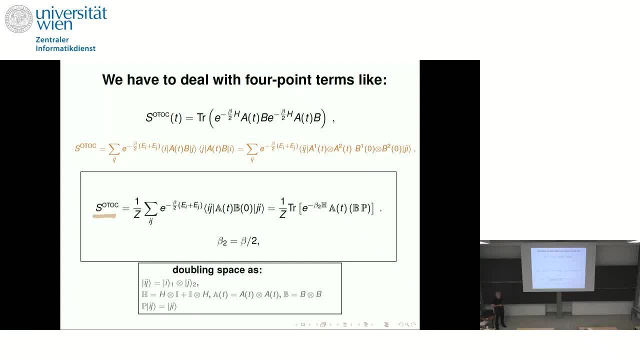 because it's absolutely nothing to do with entropy. You see, A the commutator comes from this term and this term. Then, of course, there will be a B A A B. Then there will be a B A B A. These are, there are two to. 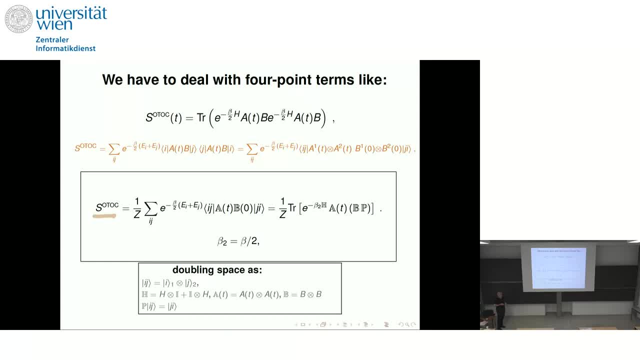 the four terms that I have to calculate. OTOC means out-of-time-order correlator. Yeah, because it's A. you're not accustomed to have time zero time T, time zero time T. This is why it's called. 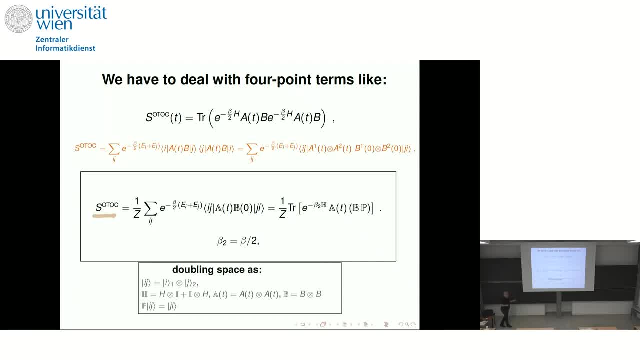 But it's one of the terms of the commutator shown here as an example only Now. so, because we don't like the four-point functions, there is a trick that exists everywhere, a bit in quantum mechanics, which allows you to go from four-point functions to two-point functions. 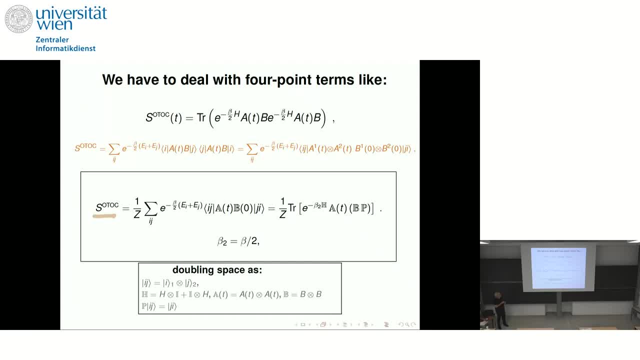 It lives in several versions, but you can if you want. this is This is what you're calculating. I just rewrote this one. But if you now make your space a product space of twice the same space, so you duplicate the space you can, and this: 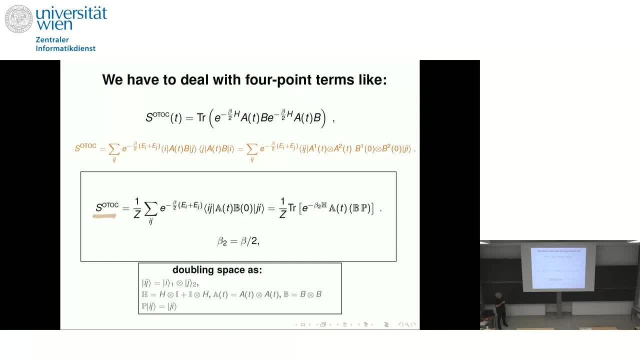 is just a standard trick. write everything as a two-point correlation. This one becomes a two-point correlation in a fatter space, which is the Cartesian product, or the tensor product of the state, or the Hilbert space with itself. Okay, This takes you ten minutes to be completely convinced. but the only morals of this is: 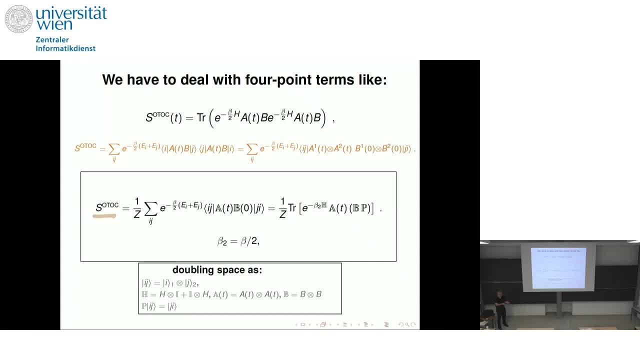 you can always take a four-point function and take it into a two-point function. Why do I want a two-point function? Because fluctuation, dissipation and such, which is what I want to use – I know it with two-point functions. 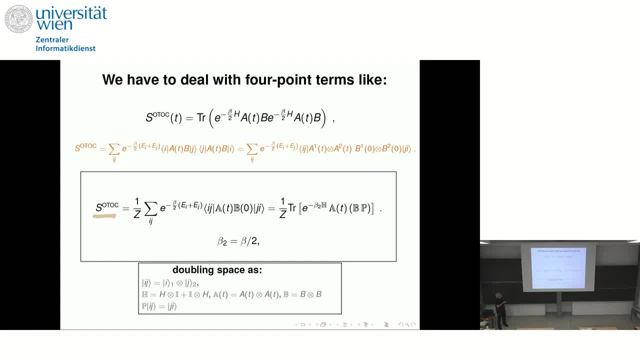 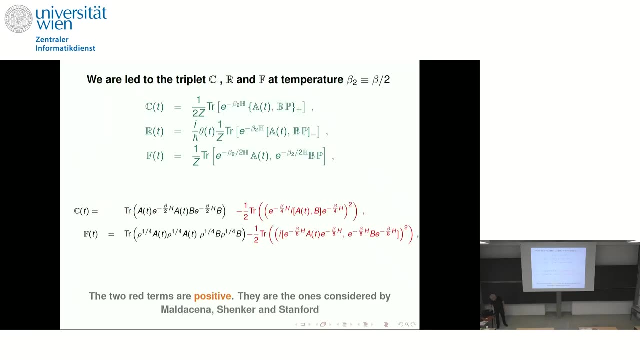 Okay, So, okay. so this same object now reads in this product space this way: P is the swap operator that takes an operator from space 2. and z to one and one to two. And now something remarkable happens. The quantities you want to calculate: 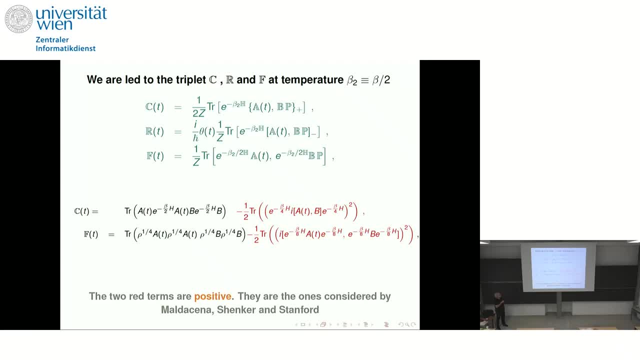 are exactly a correlation, a response and an F in this duplicated space, Miracle, miracle. So this is just the definition I did before, but in the duplicated space, doubled space. so I have anti-commutator commutator. 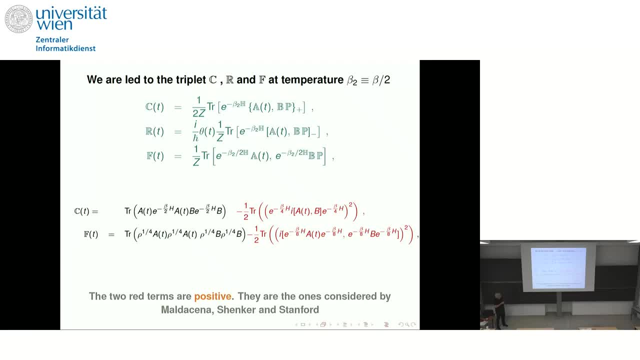 and this intermediate stuff and then, when you develop them, you get something in black which we will be neglecting. and precisely here the quantities, the version two and version three that I started with. that gives me the Lyapunov exponent. 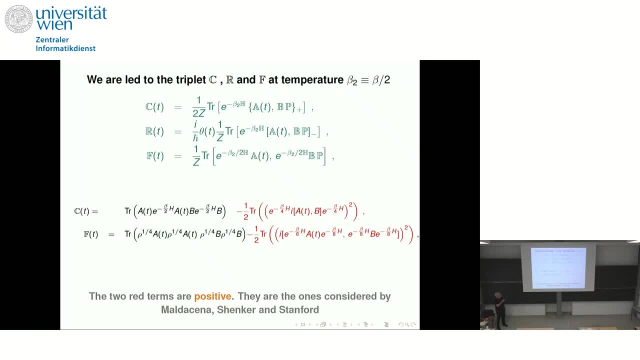 Miracle, miracle. So these two quantities are obtained from correlations and response in another space and now, but now in this space it's a correlational response and one of these split functions. Where is rho, Second line Here, Two lines below. 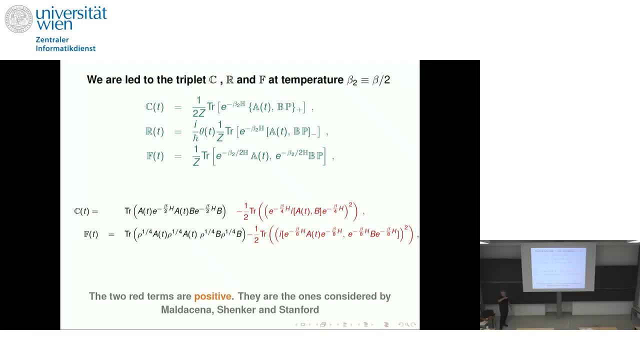 Ah, sorry, it's a Gibbs measure. It's e to the minus, so to the 1. fourth is the split one. Yes, thanks, Okay, so the quantities we wanted to prove something about. these are two versions of regularization. 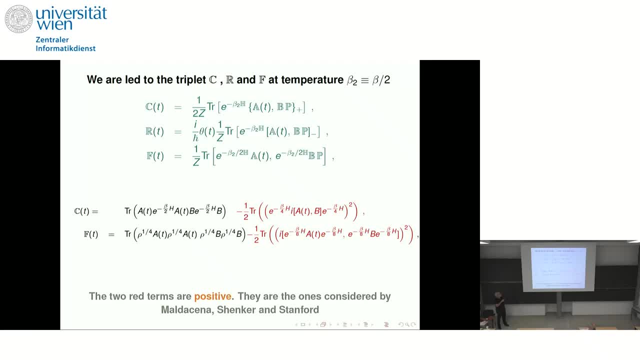 this is why I had to introduce. them are a correlation and this f function, and you could also write a response here. I didn't because we are not going to use it, but you could also. And then here you join: Maldacena, Shanker and Stanford. 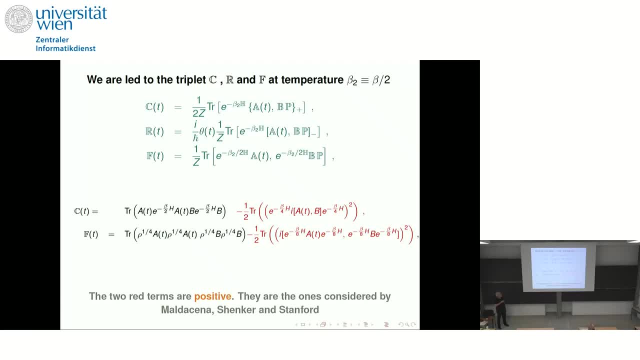 in the fact that they also use it in their proof that this quantity is a completely innocuous quantity, because it has all the things in one time here and all the things at time zero on the other side, And here too. So these quantities are not interesting. 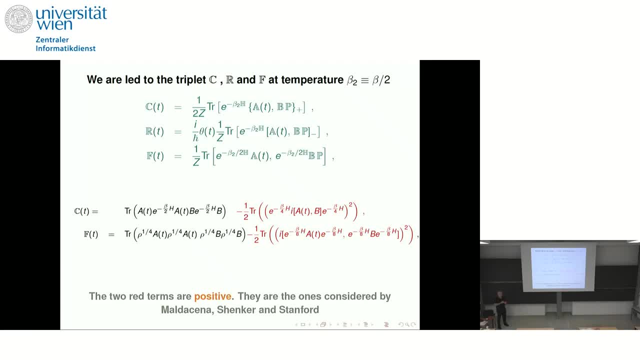 they are just a two point correlations, morally, and the idea is that they will decay much longer before the Lyapunov times that we are interested in. They also did this assumption. So basically, the red parts, which are the nice things. 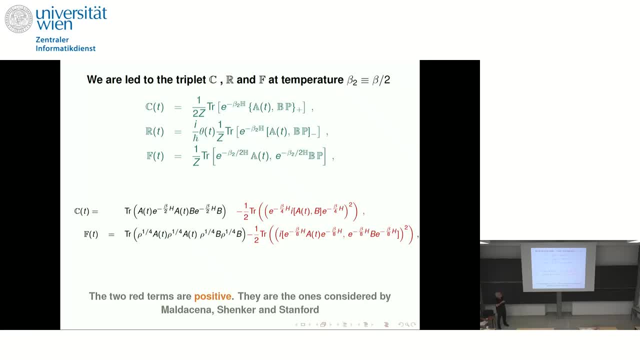 the regularized versions are a correlational response and an f. there's a third line here, in a certain doubled space, And the quantities that are regularized have the beauty that you see that they are positive, definite because they come from squares. 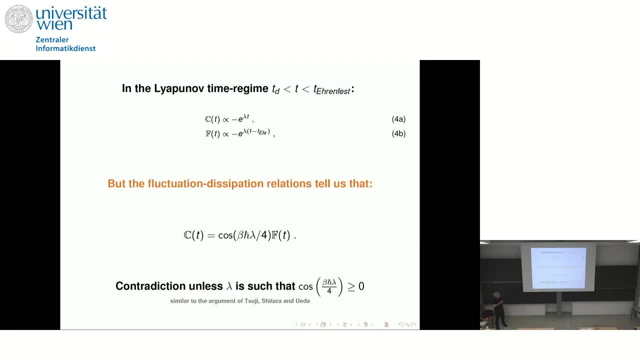 And now you're done With all this rewriting. you're done because these things grow as Lyapunov. but now, when you look at the relation between these two, because it is a c and an f there is- I told you about when you have an exponential- 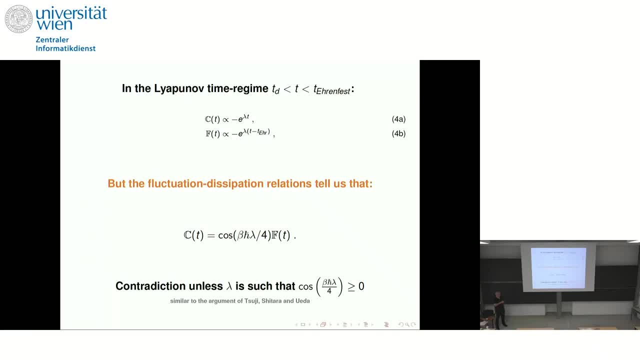 the fluctuation dissipation, quantum comes as a cosine, and so the fluctuation dissipation gives you this relation. It's the same thing I did before, but as applied to this quantity, But now we have a problem because c and f are positive. 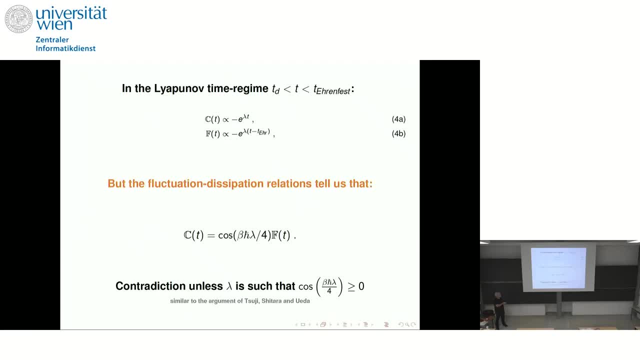 is two, So, and the cosine is not always positive precisely, and it would lead you to contradiction if this thing became negative. And if this thing becomes negative you're violating the bound. So the bound is nothing else that saying that two positive quantities. 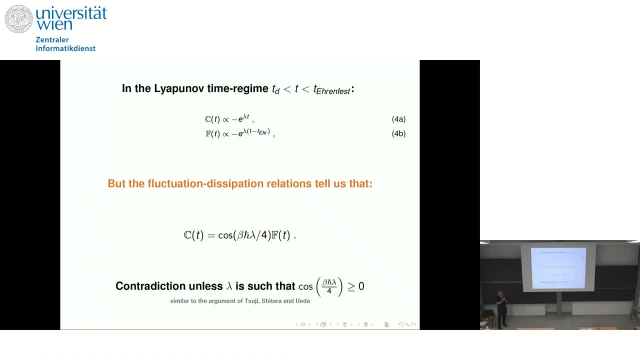 related by fluctuation, dissipation. of course the relation has to keep the positivity And because quantum mechanically there is this cosine, whatever is inside has to be smaller than pi over two. So that's a bound. Yes, it is. 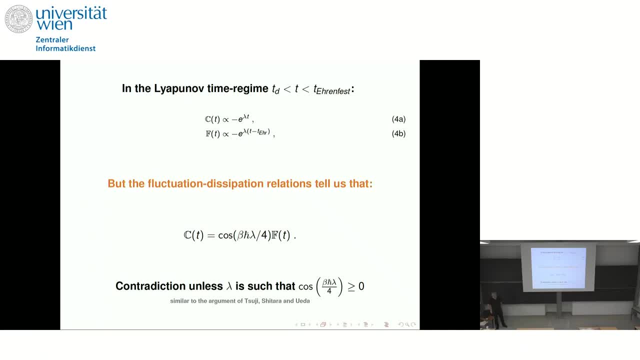 So it will be an obvious in some systems. So, precisely now that I'm here, there is a beautiful paper by Christophe and Harold Posch where they explicitly do with classically with disks and they see that with disks just by playing. 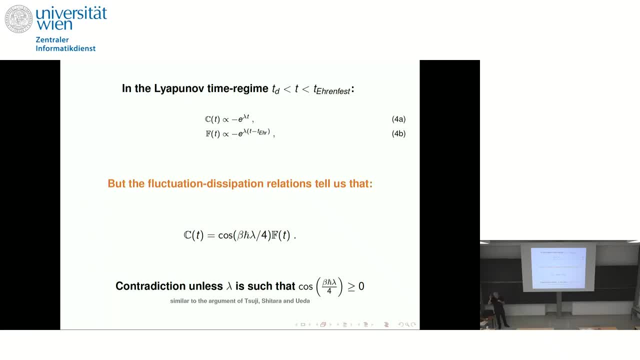 It's exactly the opposite. So everything is possible. The Lyapunov time can be larger or smaller than the collision time scale, larger or smaller. This there is a concrete example of that. But for the models that these people like- and this is an assumption of the theorem- 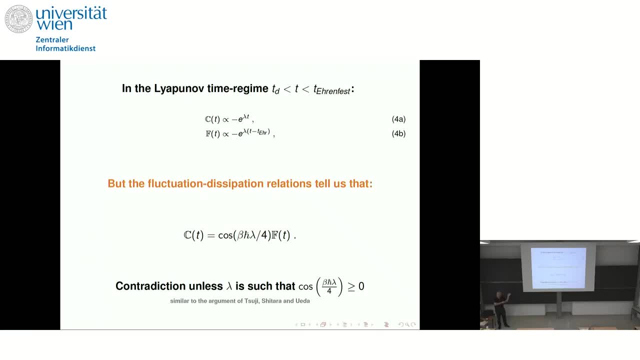 otherwise the theorem doesn't work. you have to be able to throw those bits also in the original proof. Yes, exactly. You assume that both grow and this is physically reasonable in the same way. They diverge in the same way. 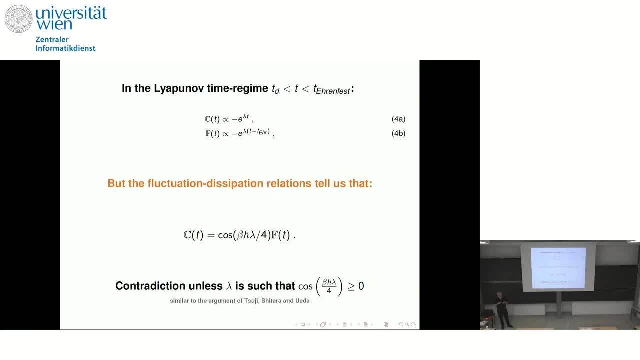 And then you conclude that you have them Exactly. And the lambda by hand requires knowing something about the system. There are many, many, many quantum systems. I would say most quantum systems don't have a Lyapunov regime, But you are bounding something so you have to assume it exists. 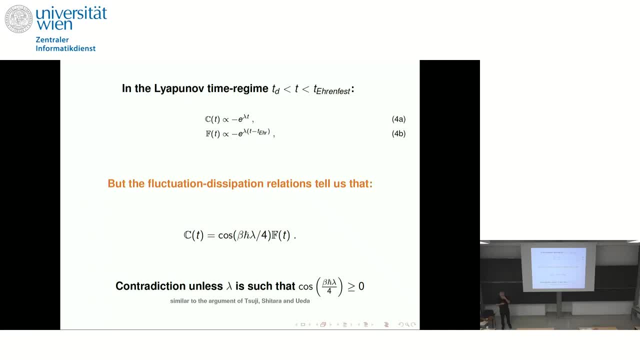 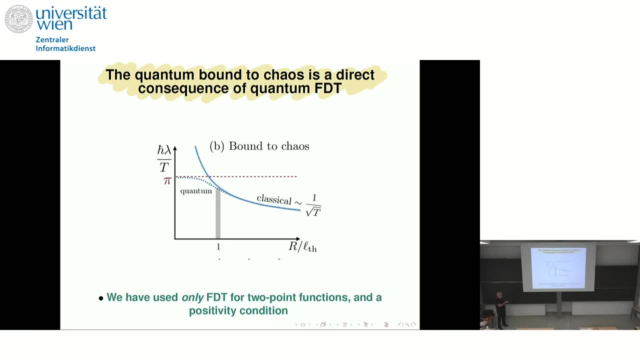 Ah, that's not stupid. There are ways You can go continuously, which I will do here, And you know that you're starting from the first Oops, The first quadrant, And then it goes up and it hits the bound there. 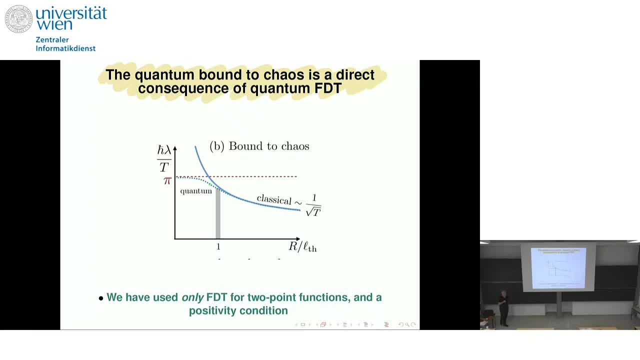 This is an argument of continuity. Somehow you have to argue something like that. Can you invent a bizarre system so that it jumps? I have never seen it. Yeah, OK, So what happens is that, for example, as you go down in temperature, so that the Broglie 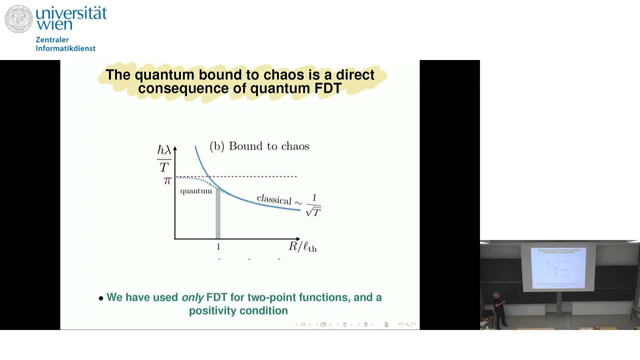 length grows in a system you hit a point at which The Lyapunov that is inversely proportional to the typical speeds boom would violate your bound. But there quantum mechanics intervenes in some way or other. But you've proven, it's general. 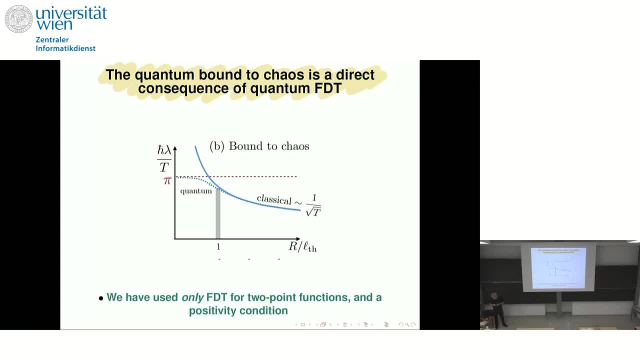 And then under the assumptions I made before- I want to underline that the assumptions are exactly the same of Maldacena, Schenker and Stalford. We didn't add anything. The only thing that we did is their analytic continuation. 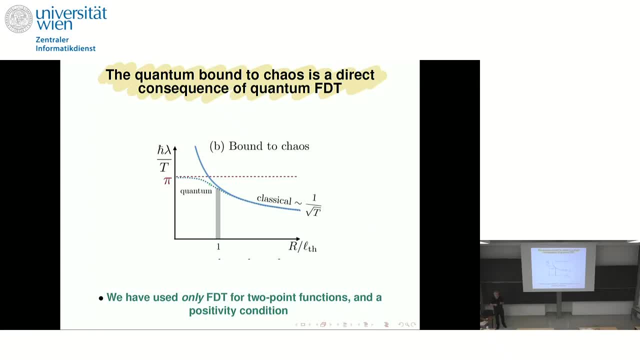 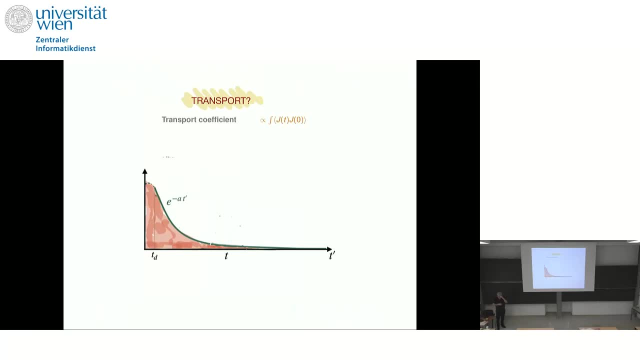 And And. a complicated argument in the complex plane for us became fluctuation dissipation Now, OK, But remember that it's not the Lyapunovs that were the original motivation, It's transport. So what about transport? I mean, this is the first instance where such a thing has been proven. 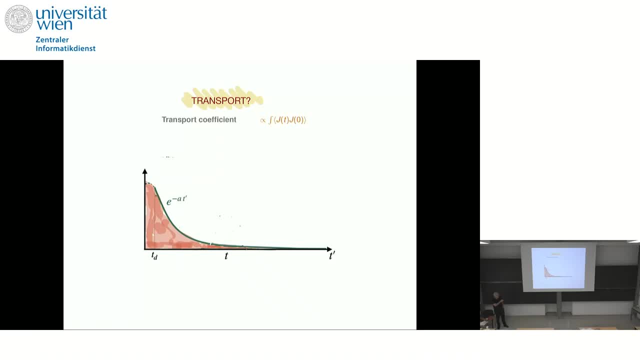 But OK, what do we do with transport? Transport, as you all know, is you have a current-current correlation And And you want the area under this curve. No, This is the integral of the current-current correlation, So you want the integral under this curve to be as small as possible. let's say, if 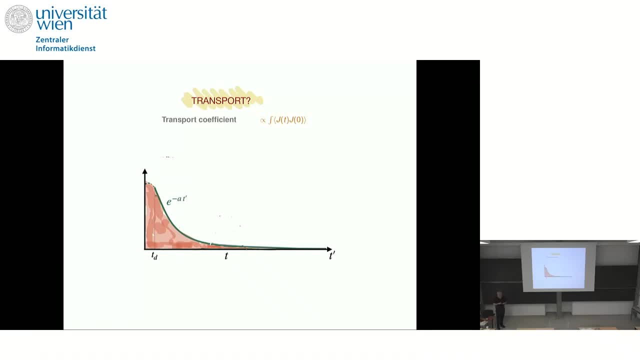 you want to show And the bound is telling you that you would like to bound it with something that has to do with h bar, And the idea is to say: this curve cannot to have a very small conductivity, sorry conductivity or viscosity. 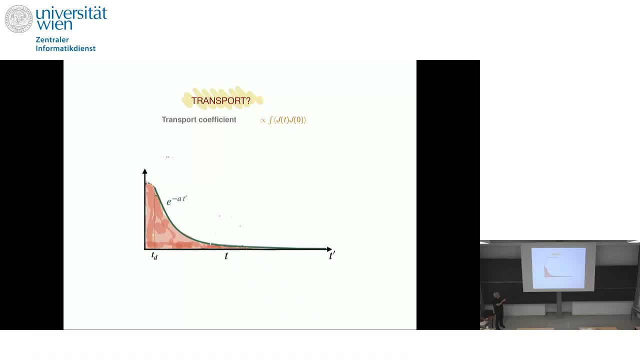 Corresponding transport coefficient. you need this curve to fall rapidly and have a small area, for example, Or arrange itself to have a small area, in any case a small integral. Now, the idea is that quantum mechanics doesn't allow you to do so. 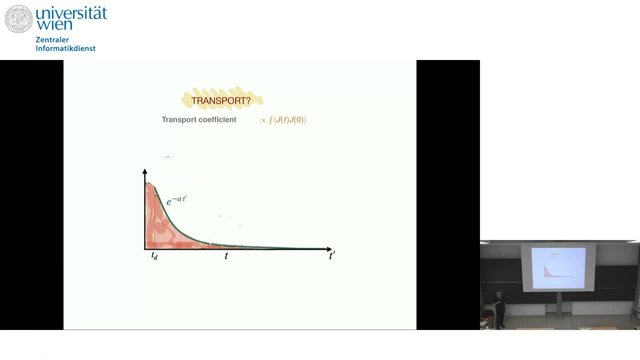 But, as I say, nobody has found a proof And it's not even clear under which assumptions such a thing would hold. However, One thing we get from here That wasn't in the original, That wasn't in the original proof of Maldacena, Shankar and Stanford: is that the crucial? 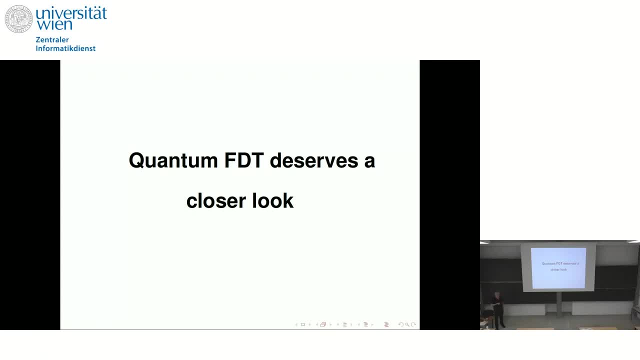 element for this to hold for everything is fluctuation, quantum fluctuation, dissipation. So it has this, yes, and I would say, but there I have a problem. I have tried to work for finite systems because they are interesting. 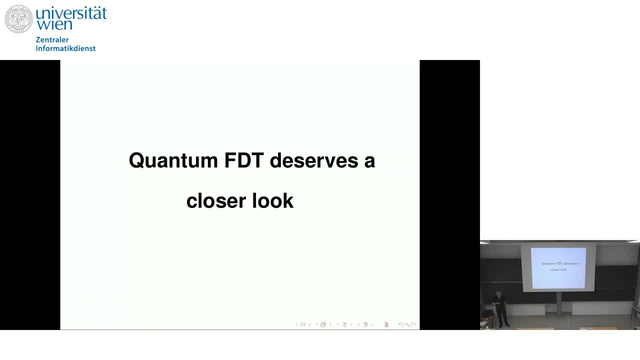 In quantum, they are especially interesting. But even saying that something decays exponentially, doesn't work or grows- Things tend to oscillate where you do. I don't know general results and I don't know to whom I should ask. But I don't even know to whom should I ask. 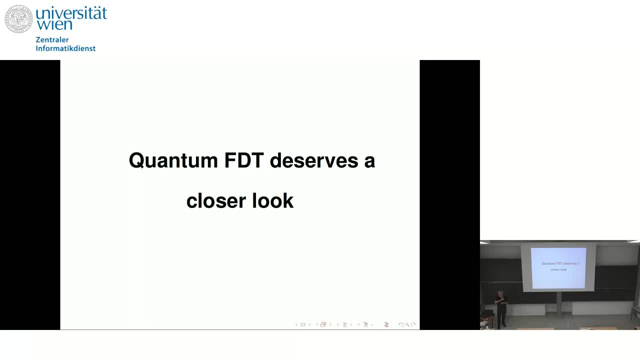 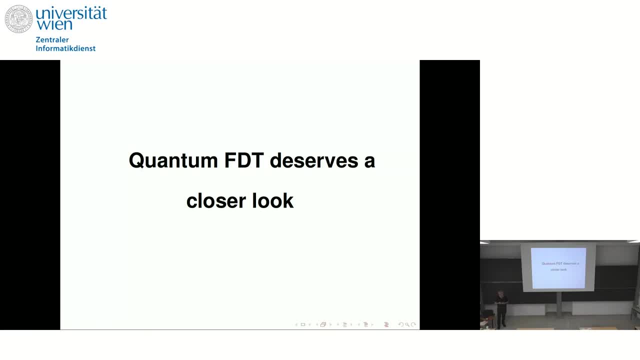 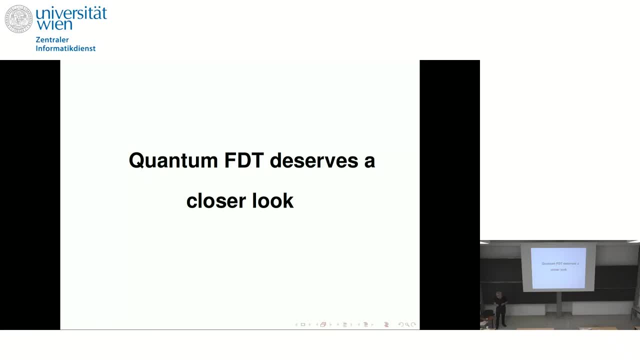 And this brings us to another thing. Remember the bound I put on viscosity, which we don't even know if they exist, but the one that was postulated is the viscosity divided by the entropy per unit particle. Yes, What do I know? I mean the bound could have something else below. 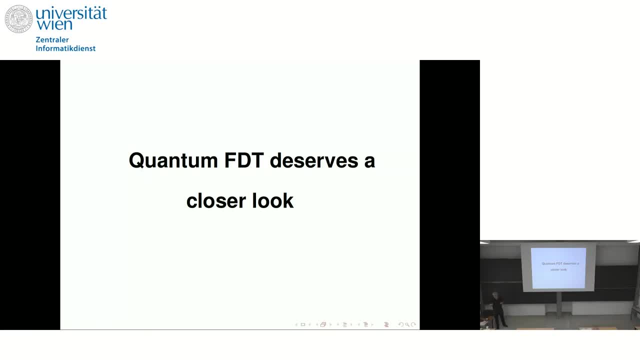 So what is in the proportionality constant? Even that is not clear. So is there a bound? Question one, Question two: what is the exact form of that bound? What is the proportionality constant? So somebody who believes blindly would answer to you: yes, but you know when it's an insulator. 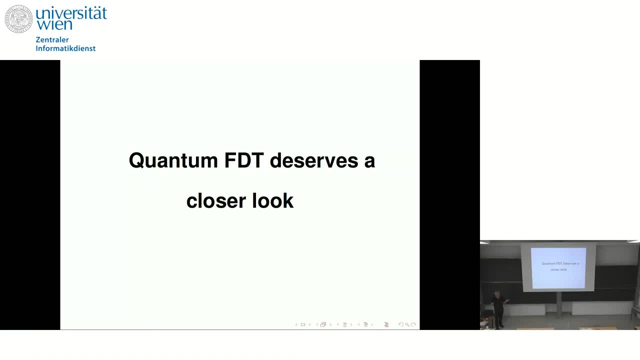 there's a pre-factor in the whole thing that will go to zero. I don't know. But the tough part to prove is the area. no, The other part is supposed to be an equilibrium quantity, So quantum FDT deserves a better look. 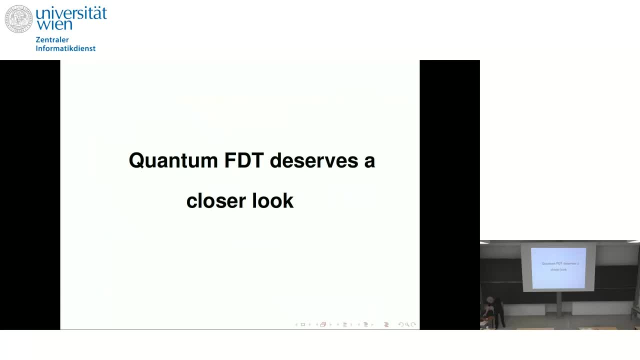 And what can we find? Because, remember, the point is that the transport is a question of two-point correlations. It's really a question of two-point correlations, not four-point correlations. We managed to convert a four-point correlation into a two-point correlation. 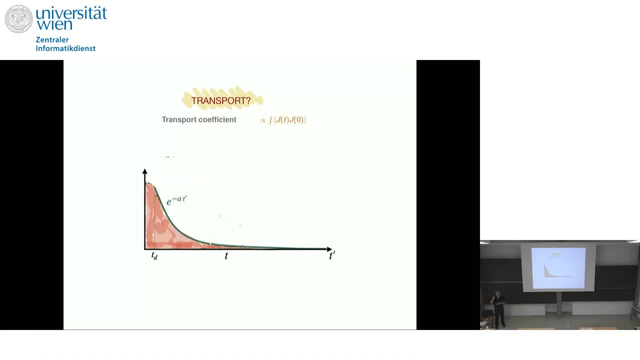 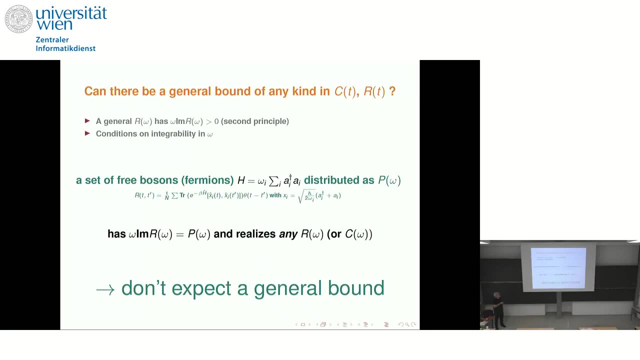 but in the process we found that two quantities were positive, definite, and that was crucial for us Here. you don't, in general, have such things. So what do you do? Well, first thing you can convince yourself is that just by considering a pile of oscillators. 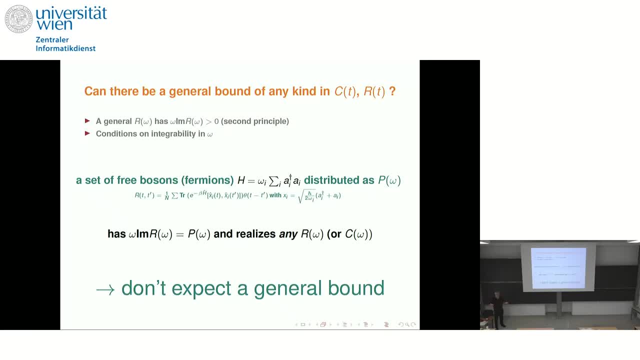 just independent oscillators and different oscillators with frequencies that you like. you can always do that system. You can convince yourself that you can do that. Essentially, you can have the correlation and the response that you want. You can construct any. there are basic constraints on signs. 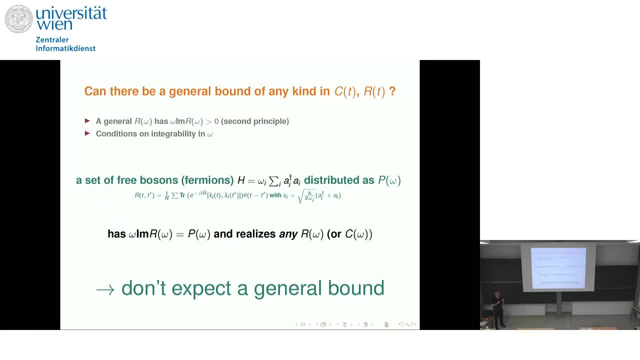 but other than that, you can construct the correlation and the response that you like just by putting correlators one on top of the other. yes, So there can be no bound. that is general for correlation and response, because I can you give me something you like. 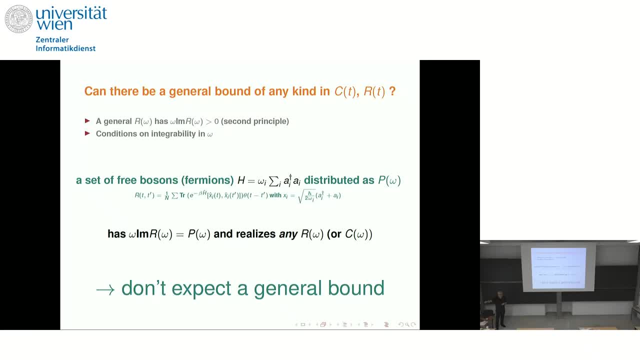 and I make it for you just by piling oscillators of appropriate frequencies. So surely there is no bound on the decay, a universal bound on the decay. So something more has to enter the game. So the first moral is: don't expect a super general bound, something you will have to put. 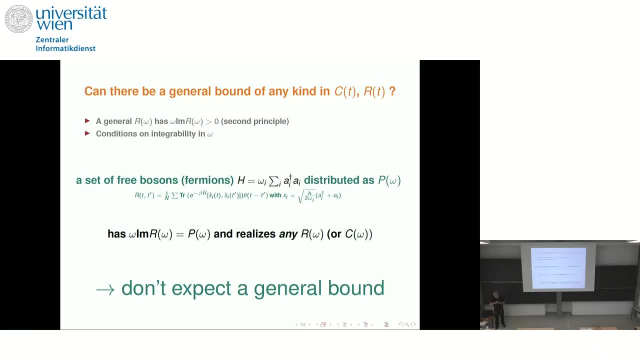 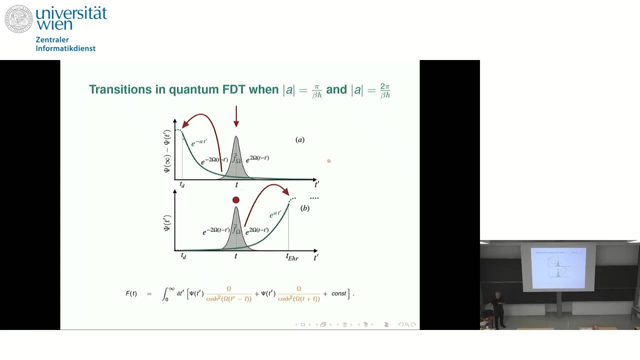 So maybe Abhishek, your insulator, will be out of my bound the day we will find it? no, But I would like to emphasize the basic mechanism. Remember that I told you that fluctuation-dissipation, this function that goes from, takes you from one place to the other. 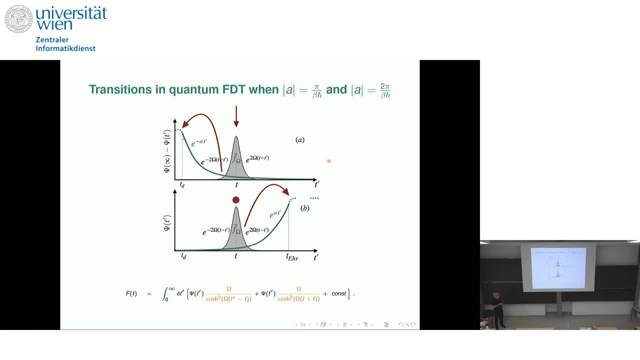 is a convolution of your correlation, or your response in time with this one over cosine squared, hyperbolic cosine squared, So it acts as a blurring function. So this already seems to be telling you that if your response had, you know, a very steep change. 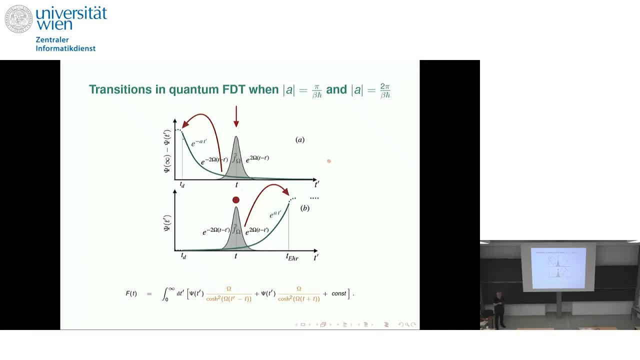 somehow, when you go to the correlation, you will lose them Because, and vice versa. So there is this blurring that seems to be at play, or at least one of the leads that we are trying to follow. Another thing that I find is quite fascinating, and I don't understand the deep meaning of this: 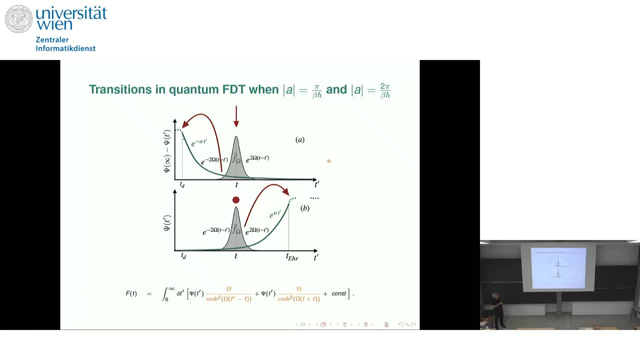 is that if this is an exponential that falls, if it falls fast enough- and you are convoluting with this- if this exponential of the system fell more rapidly than the Planckian rate, the Planckian time, then this convolution is no longer dominated by. 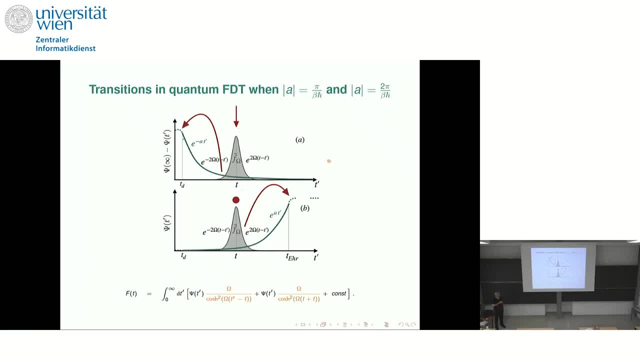 around this point. It is dominated by the very short times. So if something falls super fast- faster than Planckian- everything that happens at long times is dominated by the short times. What is the meaning of this? I don't know. 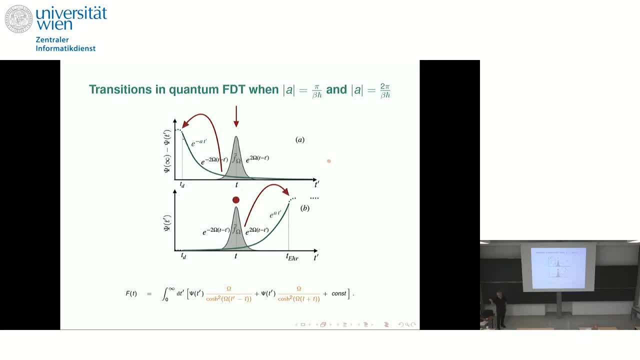 I mean, when you talk to conformal people, they are happy because in their stuff short and long agree. but for non-conformists this is strange And in the case of something growing, the opposite happens If the growth is where. 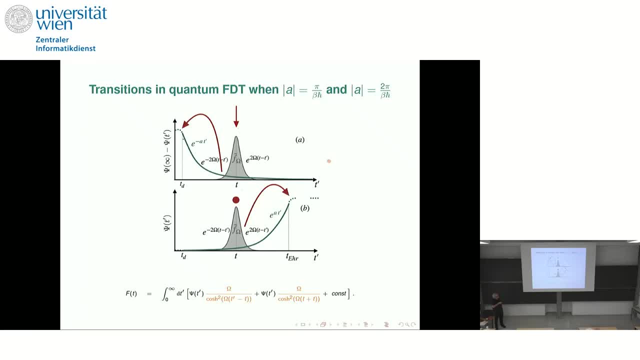 Super Planckian, then again, this thing is the one that late times dominated. So I don't know. These are all leads that we are trying to follow. Of course, if this is a smoothish function and you're going to a narrow case, 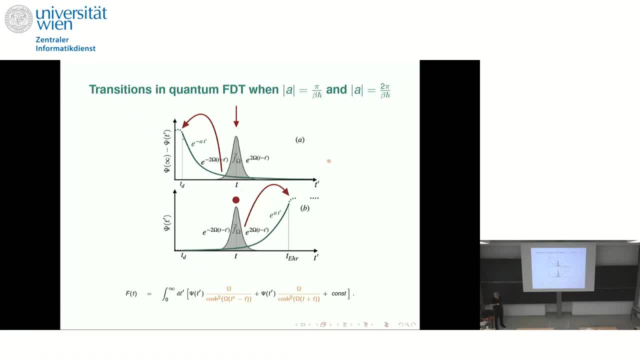 or you're going to the classical limit. convoluting with this Gaussian is the same as essentially evaluating in the point- and you tend to- either the classical fluctuation, dissipation or some little fluctuation thereof. some correction, Okay, this is the kind of thing that is interesting. 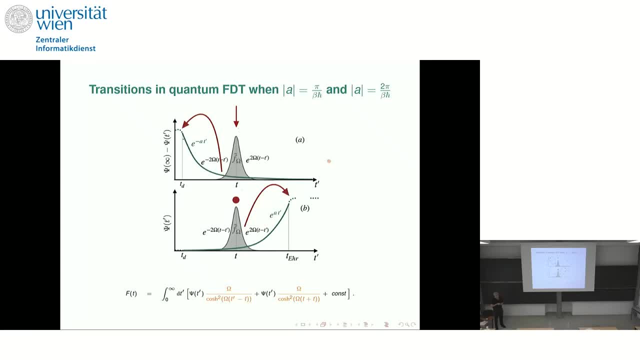 because it gives us a perspective of what fluctuation, dissipation does. Will it lead to some form of bound to transport coefficients? We don't know. There are, people are divided on this, but we don't know. Is there a true? and if there is a true one for transport?